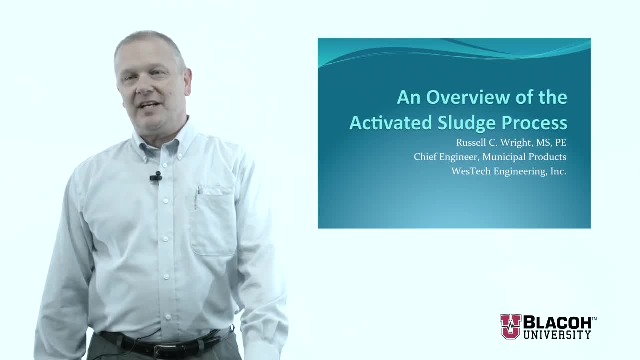 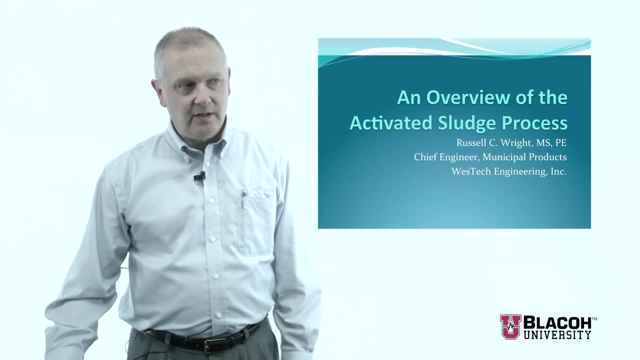 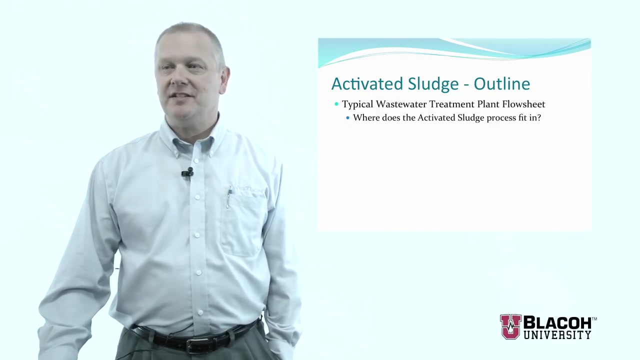 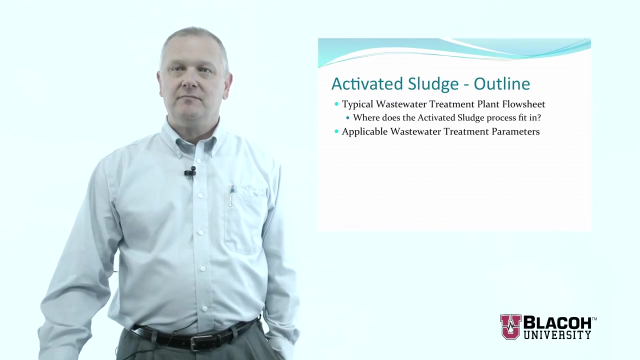 classes in wastewater treatment, as well as a master's in business administration, And so with that, let's proceed. We're going to talk today about, first of all, where the activated sludge process fits in a typical wastewater treatment plant flow sheet. We will then go over some important wastewater treatment parameters, or 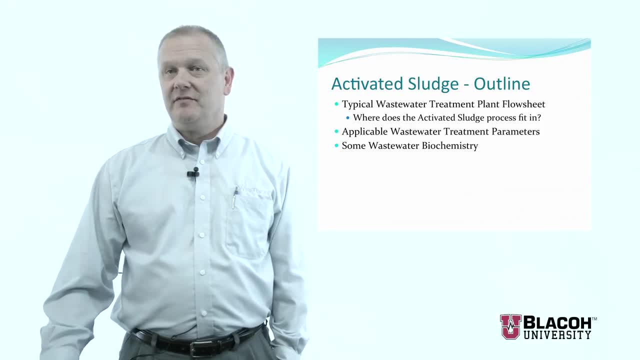 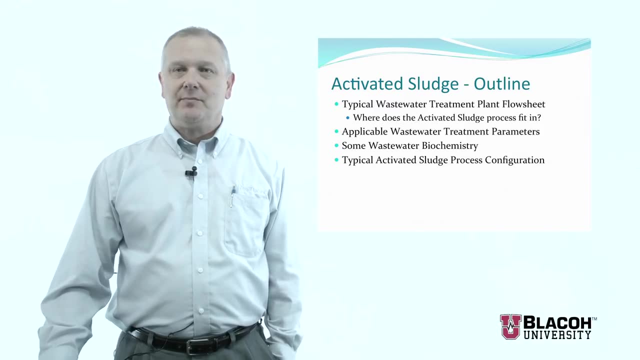 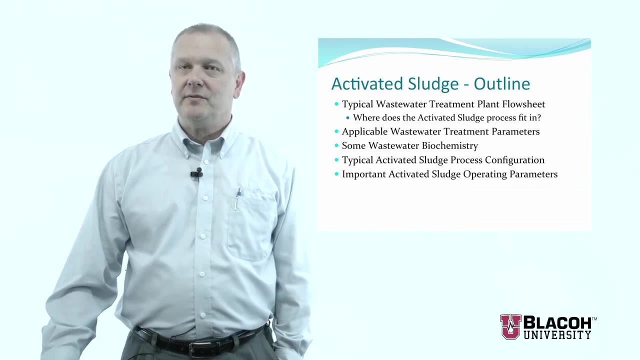 criteria that deal with the performance of the system. We'll do some very brief biochemistry and then we'll get into what a typical activated sludge system looks like, how it's configured. We will move on to talk about some important parameters that are used to operate an activated sludge. 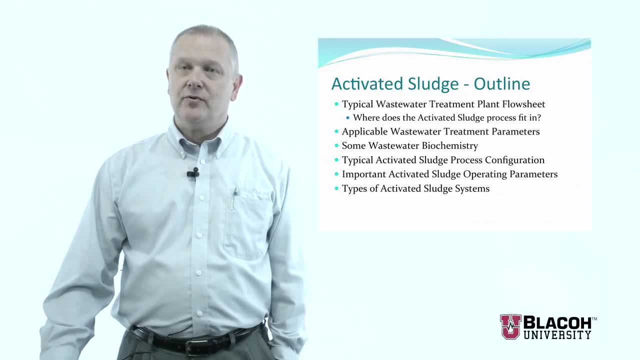 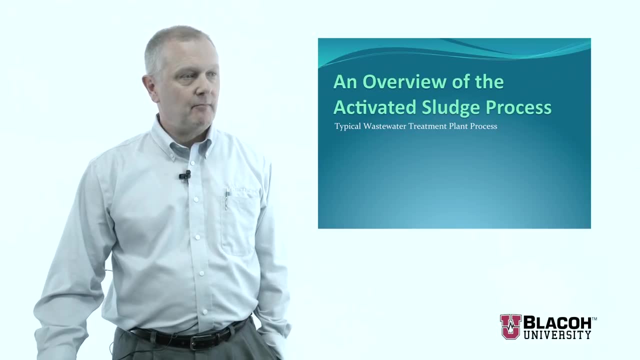 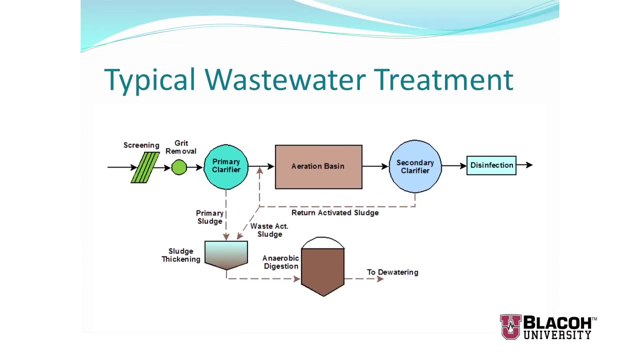 system and then, finally, we'll go through some different types of systems in actual treatment plants. So a typical wastewater treatment plant flow sheet looks something like this. There are many variations, but this is a very typical flow sheet. We start out with screening. This is designed to remove. 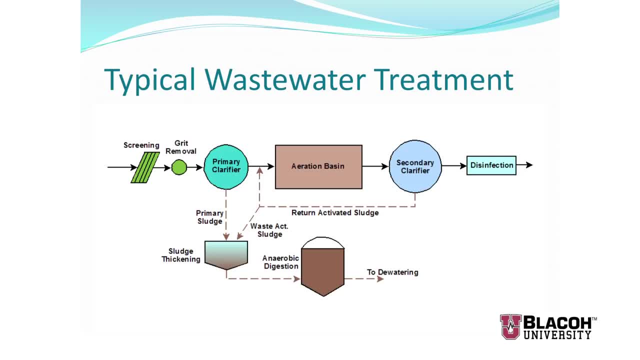 rags, paper, plastic products from the sewage coming into the plant. I even had an operator tell me a mattress came floating down the sewer one day. We want to screen this kind of stuff out before we get into the rest of the plant, And so 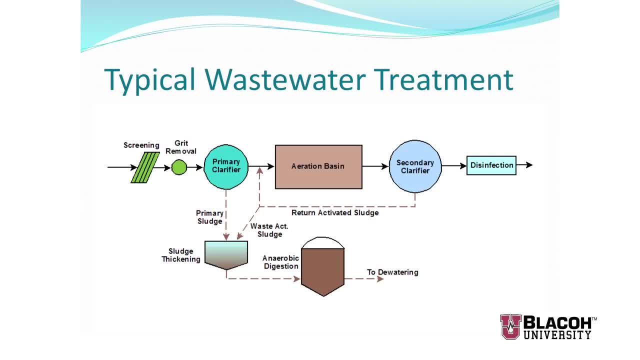 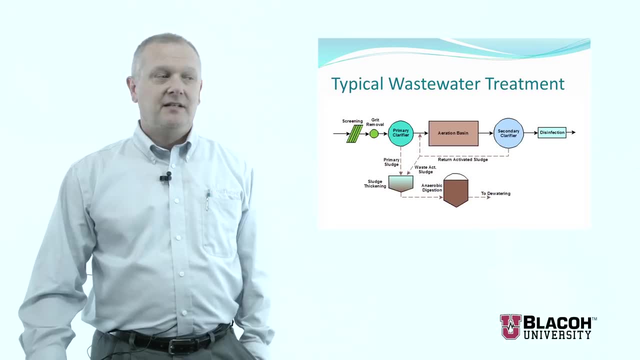 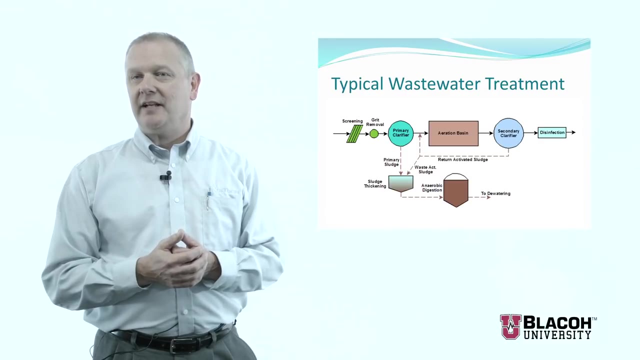 there's always some type of a screen at the head of the plant. Following the screening is grit removal. Most sanitary sewers are made from concrete pipe And as concrete wears you get sand particles, fine grit that moves down the pipe and into the treatment plant. That grit is a problem If you run grit through a pump. 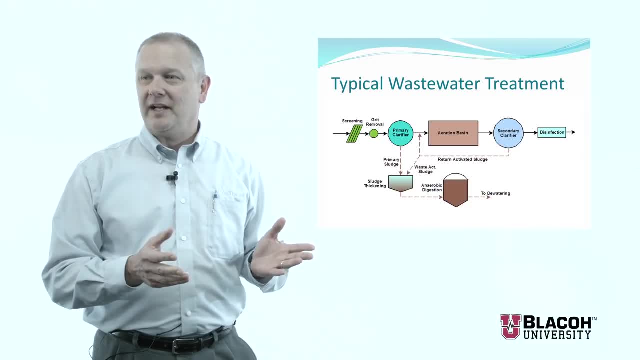 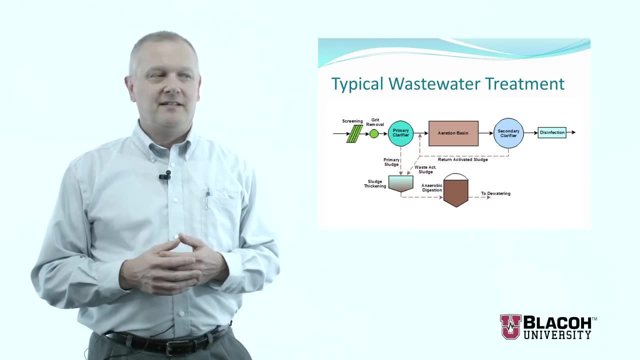 you'll wear the pump out very quickly. There are a lot of pumps in a treatment plant. That grit can also settle at places in the plant where you don't want it to settle and cause problems. So we take the grit out up front with some simple tanks and 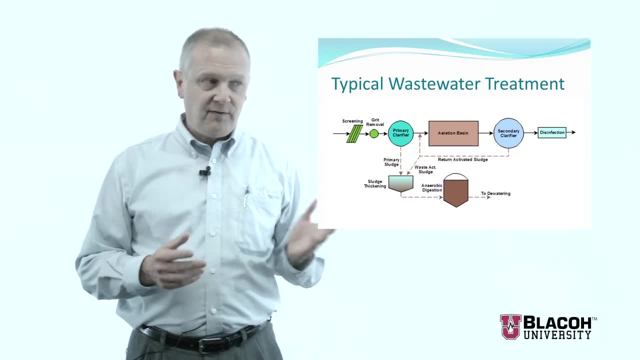 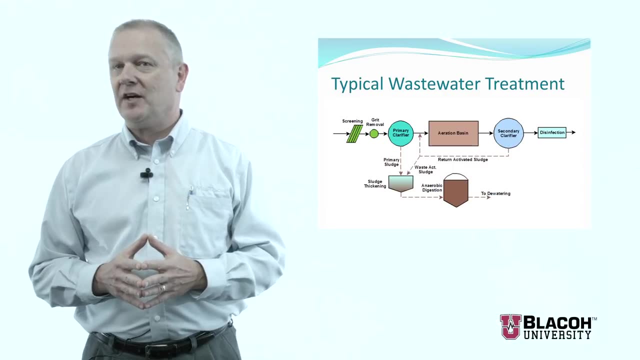 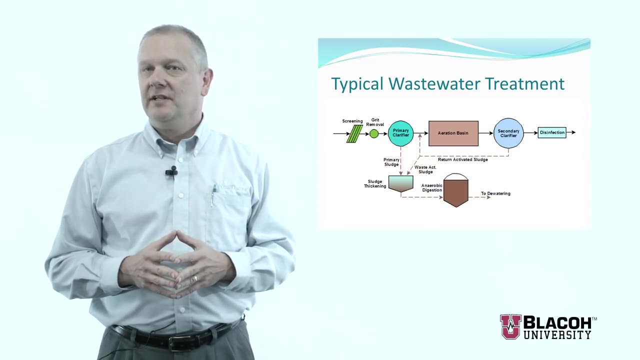 mechanisms that remove the grit Following. that is what we call primary treatment or a primary clarifier. Not all treatment plants have primary clarifiers, but any treatment plant bigger than about five million gallons a day typically has primary clarifiers. All that is is a large basin that the liquid. 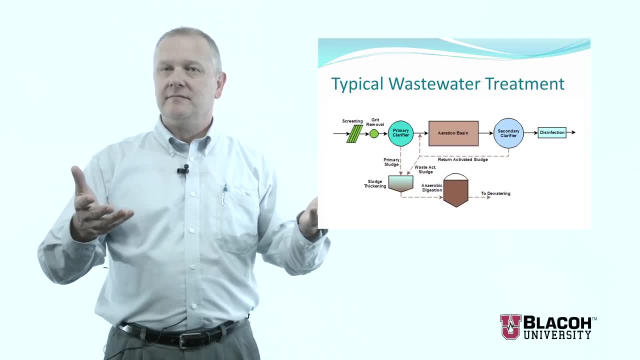 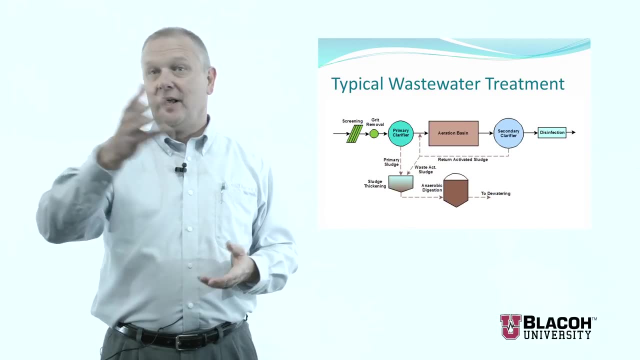 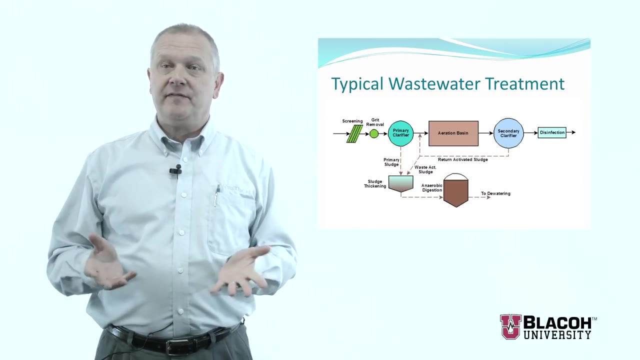 flows into And any solid material in that waste stream will settle to the bottom of the tank where it can be collected and removed, and the clear- relatively clear- liquid then flows on into the rest of the plant. That removes about fifty percent of the contaminants in typical sewage And it's obviously very 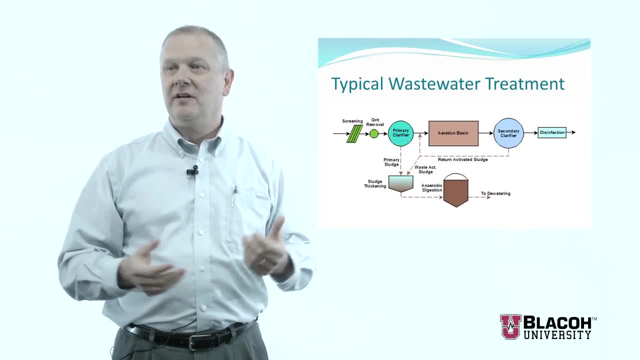 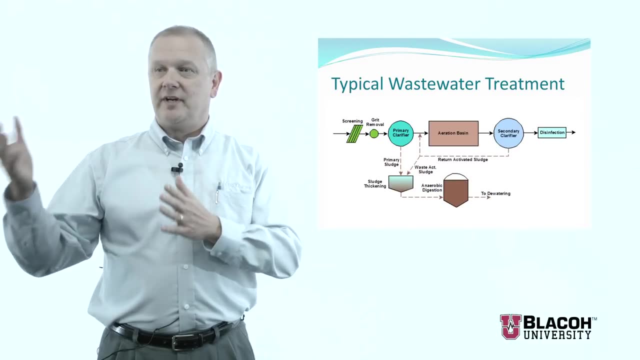 inexpensive: All you need is a big tank. It doesn't take a lot of power or energy, and so it's an important part of just about every treatment plant treatment process. But what do we do with the rest, The part that won't settle the? 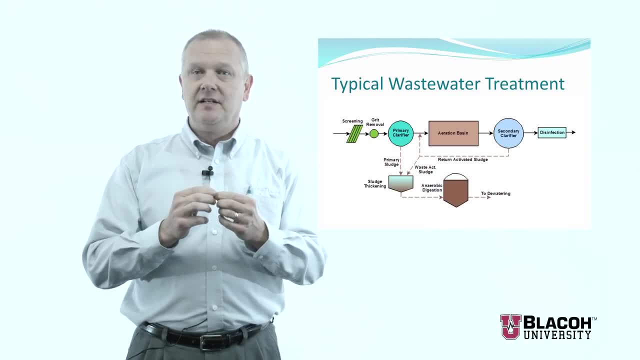 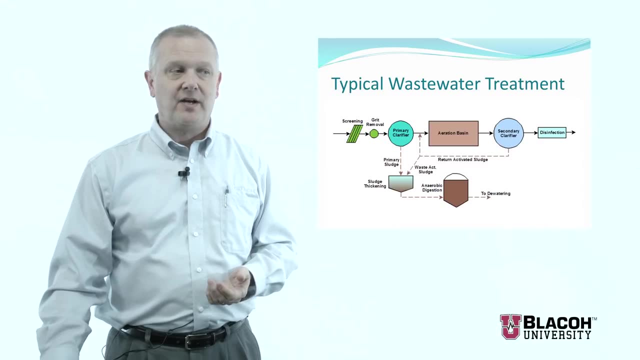 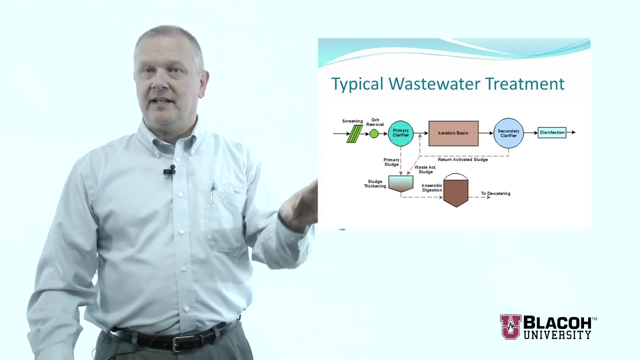 part that's dissolved in the wastewater or is very, very fine particulate. That's where the biological secondary process comes in, and activated sludge is the main process that's used throughout the world to accomplish this. I will explain more exactly what's involved. 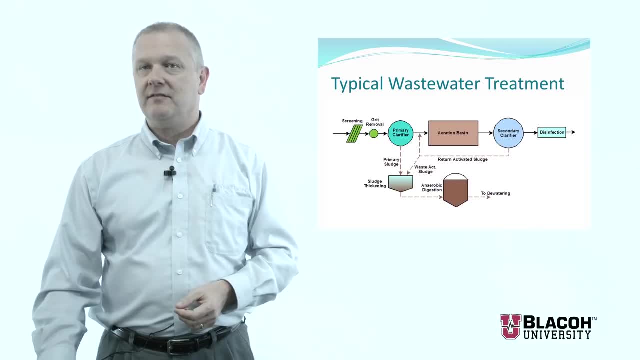 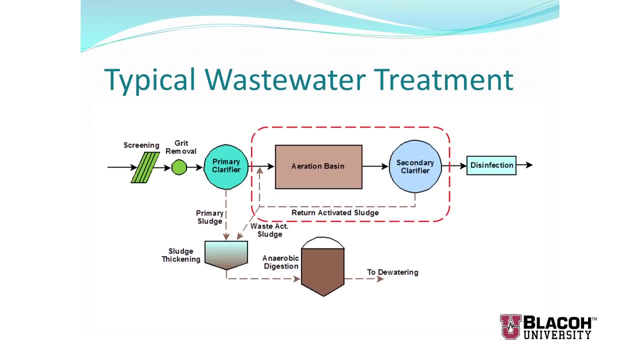 in that system. but you can see in the diagram where that activated sludge system is located. It consists of a large aerated basin and a clarifier and a recycle stream. Following that, the liquid has been cleaned quite well and all that's left is disinfection. where 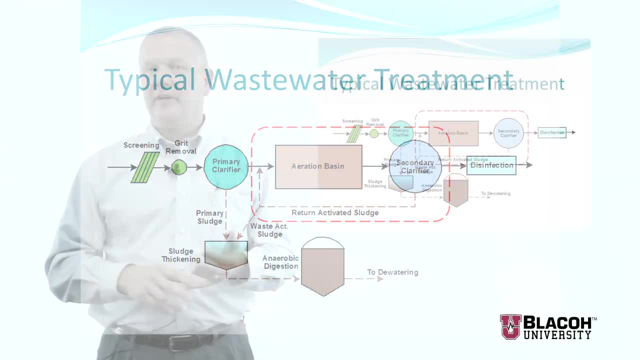 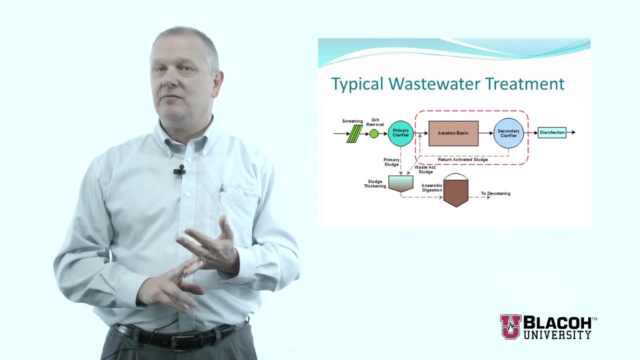 we kill whatever germs are left using chlorine or ultraviolet light. Many treatment plants are going to the UV light disinfection now because chlorine is hazardous and difficult to work with And the UV disinfection is sort of like giant high strength tanning beds. You run the water. 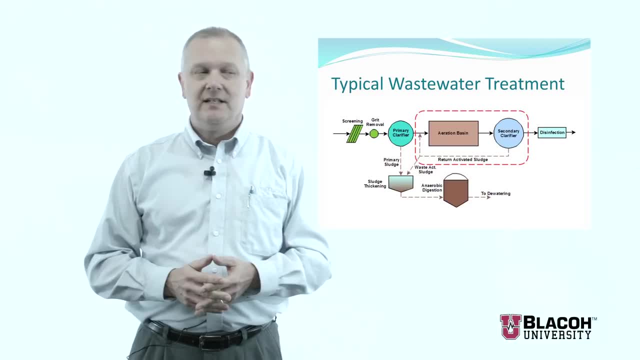 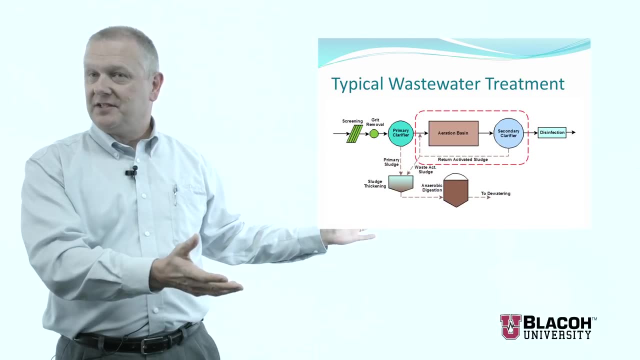 through there and it actually will kill the germs that are left in the wastewater On the lower part of the flow sheet. you can also see that we have to handle the solids that settle. The solids go into a thickening stage and then into a digestion stage where 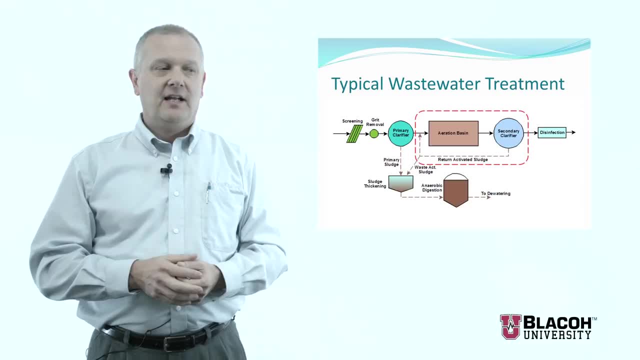 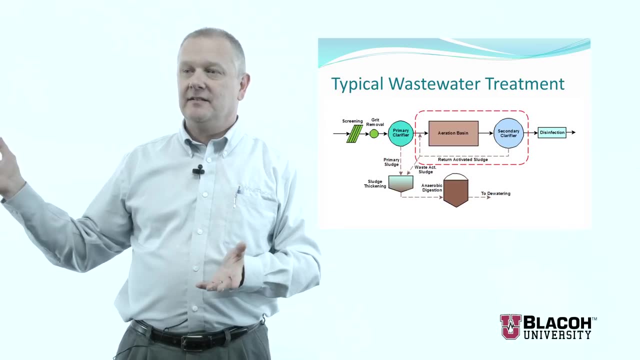 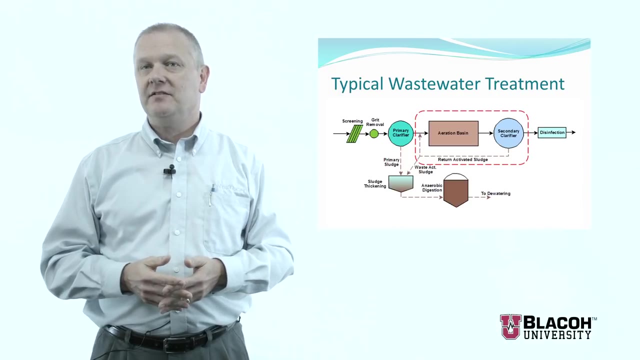 the goal is to reduce the volume of those solids. And then it's dewatered and it can be composted to create fertilizer. It can be directly applied on agricultural land non-food crops. There are a lot of ways that plants deal with the solids that come off of the treatment process. 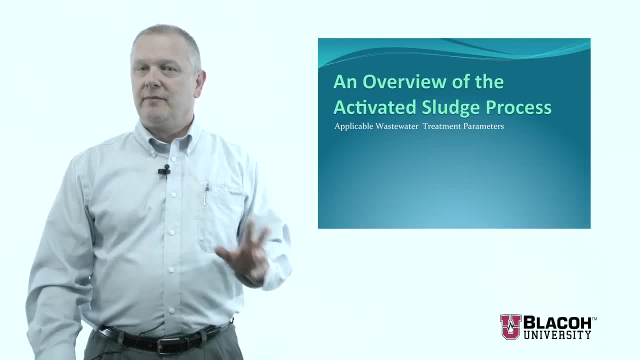 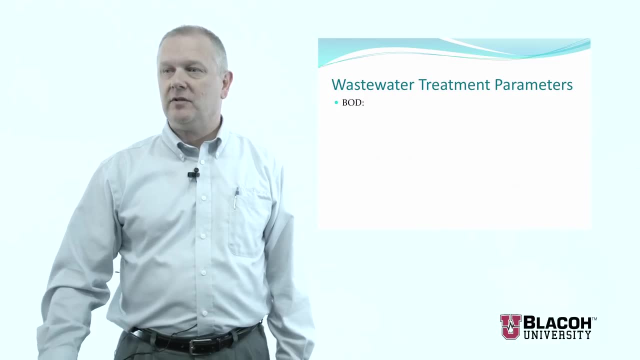 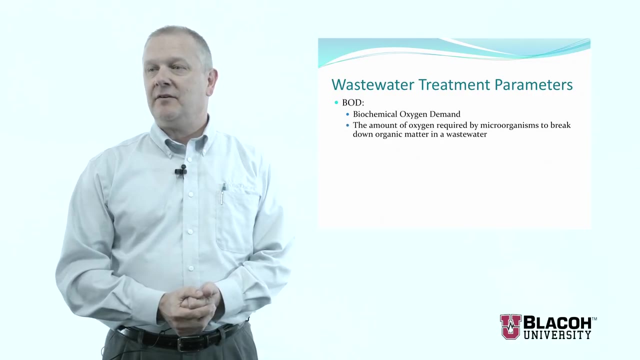 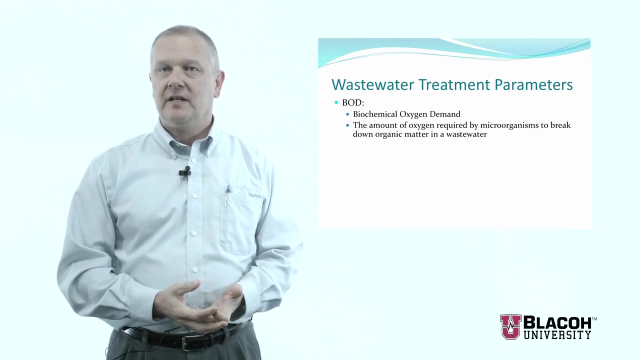 A couple of important treatment parameters that we want to talk about. The first one we call BOD. That stands for biochemical oxygen demand. This is a measurement of the amount of oxygen it takes for microorganisms to break down the organic material in sewage. The microorganisms 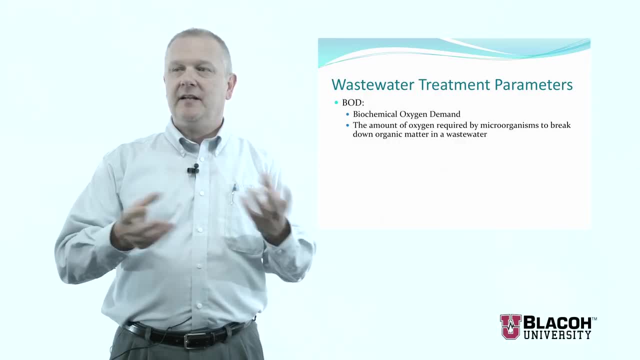 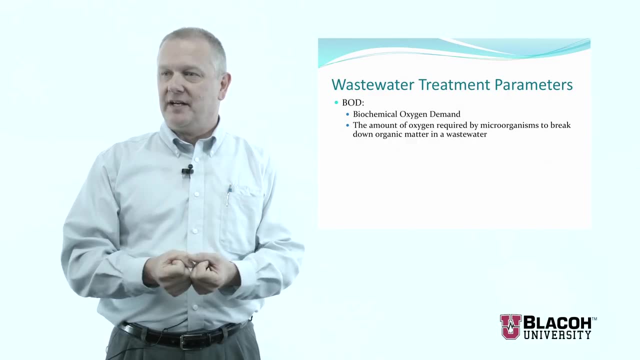 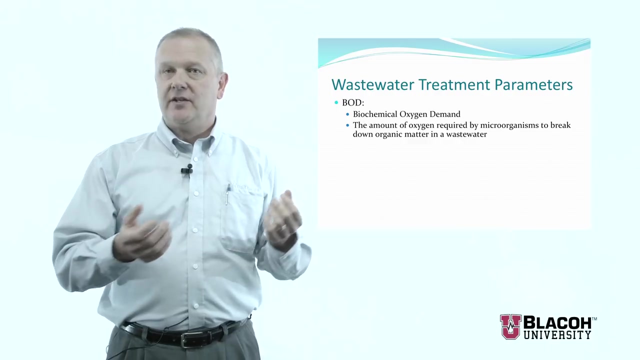 in the natural environment will do that. They will feed on any dead animal or any waste or something like that organic matter in the environment. You know bacteria break those down And these bacteria need oxygen to live. And so if you put some waste material into a stream, for example, and microorganisms begin. 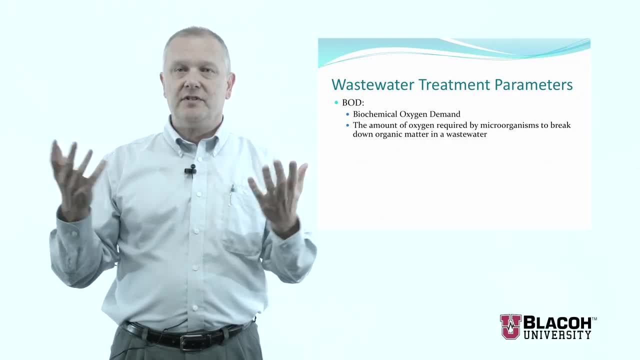 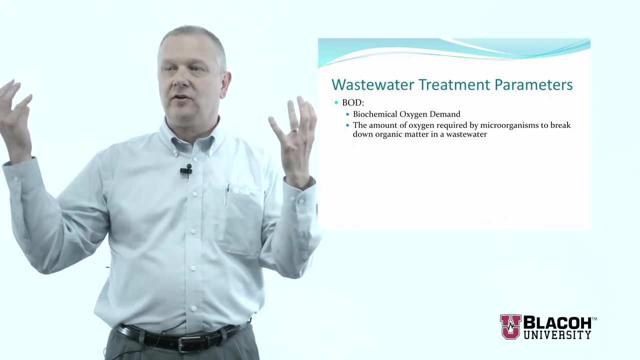 to feed on that and they use oxygen as they do. so they respire like we do. they will grow and multiply, And if there's enough waste there, they will grow and multiply to the point where they suck all of the oxygen out of the water. That's bad. Now you have a dead 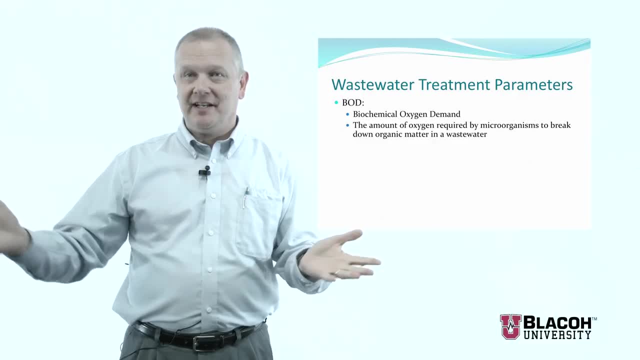 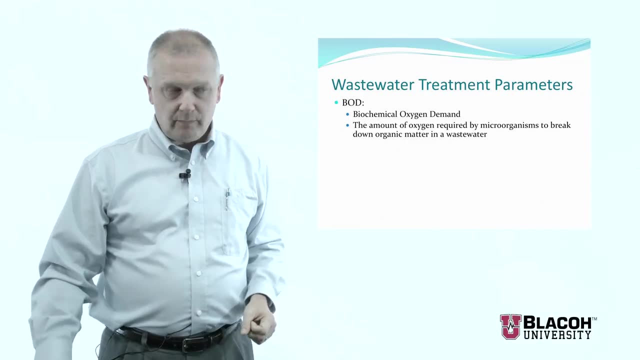 stream or a dead lake, It turns black. Everything in it dies. Not good. That's why this is an important parameter. The actual test we use is called a BOD-5 test, And the way the BOD-5 test is performed is. 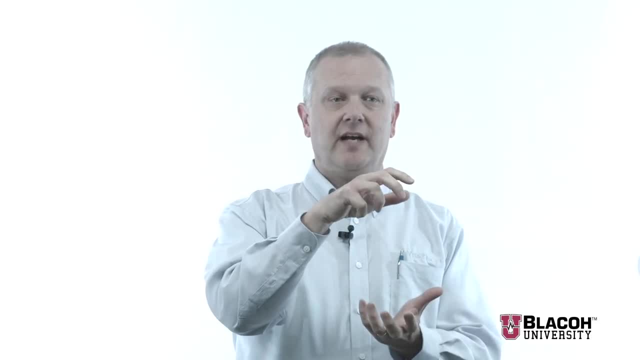 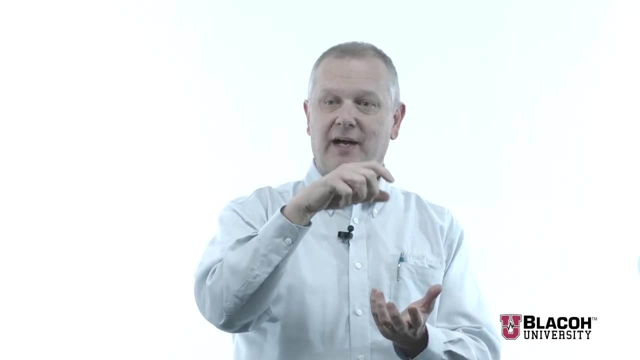 we take a bottle with water in it that has been aerated and we measure the oxygen concentration in that water. We add our waste water sample and a seed of microorganisms that will break down that waste. We seal it tightly and we put it in a cabinet. 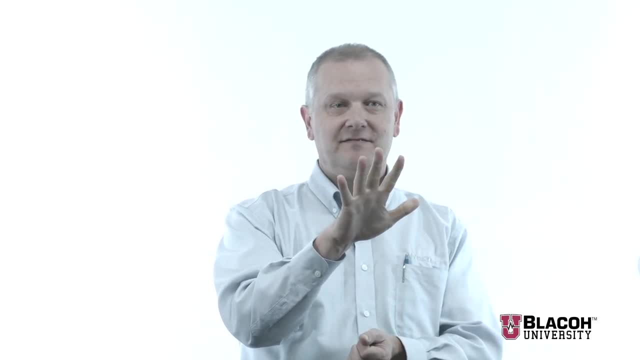 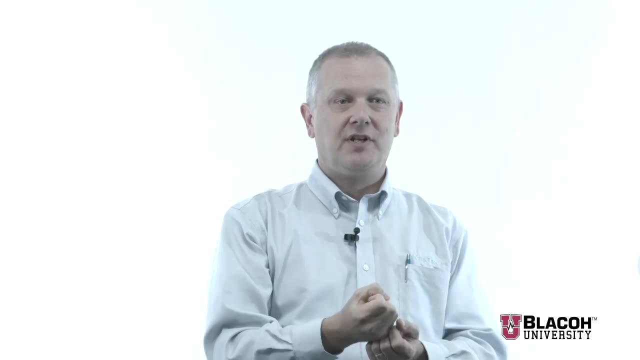 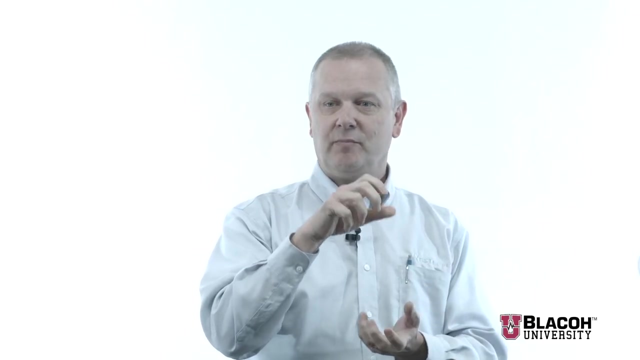 at 20 degrees centigrade for five days. We pull it out, We measure the dissolved oxygen concentration. We know how much oxygen was used up And that becomes then a measure of the biodegradable organic material that was in that waste water that we put in the bottle. 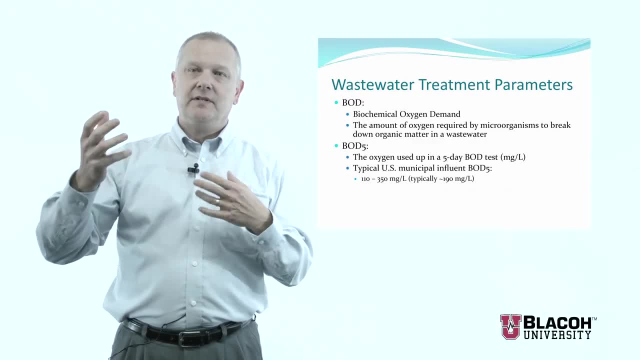 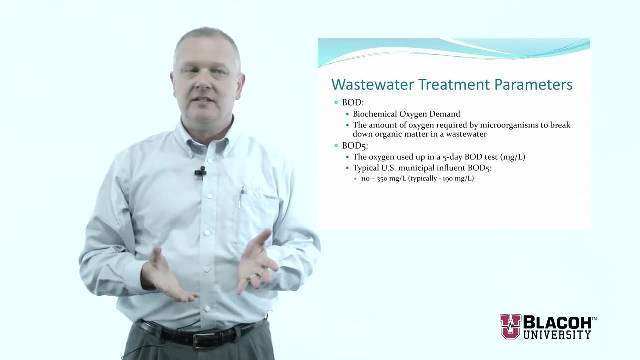 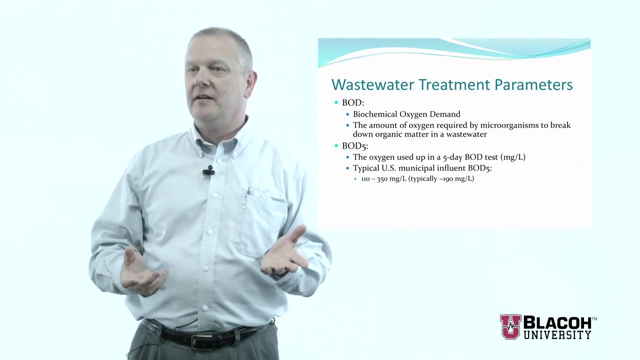 Typical influent BOD, that is, the BOD that's measured on the influent to a treatment plant, is typically around 200 milligrammes per litre, Anywhere between 100 to 350, depending on the type of community, whether their industry is contributing or not. That's a very typical. 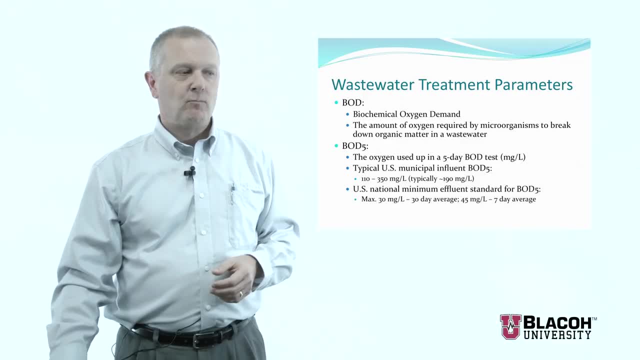 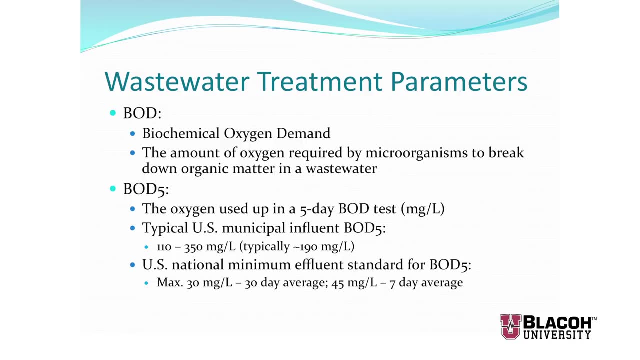 kind of number. Ok, Um, the US national minimum effluent standard on the far end of the treatment plant says that the treatment plant cannot put water into a receiving body that is more than 30 milligrammes per litre liter of BOD on a 30-day average, 45 for a 7-day average. Now, that's the US national. 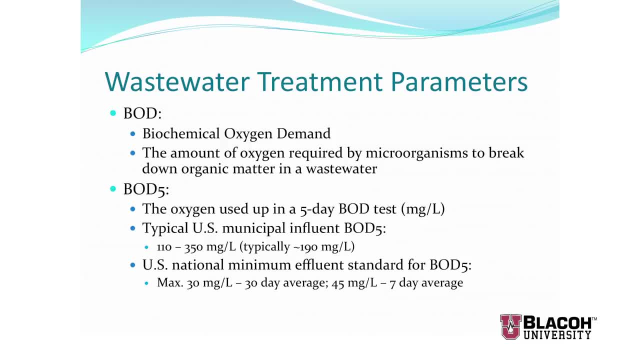 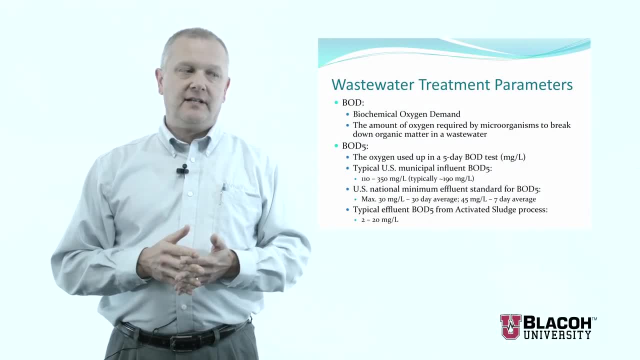 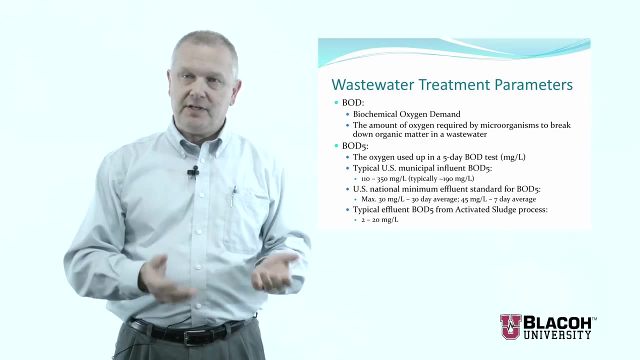 minimum part of the Clean Water Act of 1972.. But there are many state and local standards that are considerably tighter than that, and so the activated sludge process is helpful, because from that process typically we can get BOD down typically in the single digits. 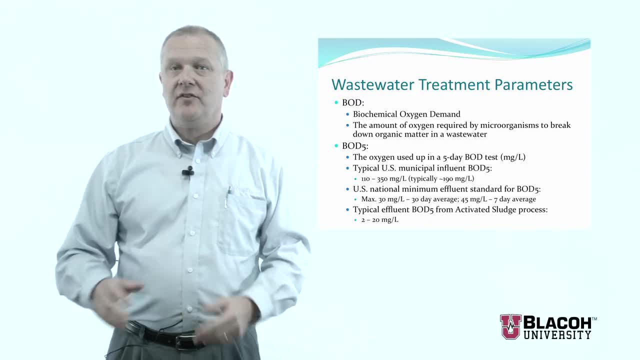 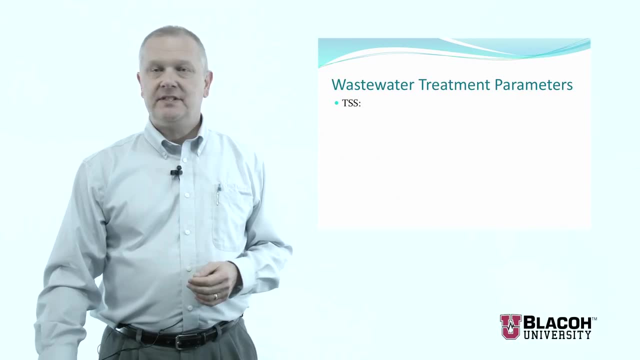 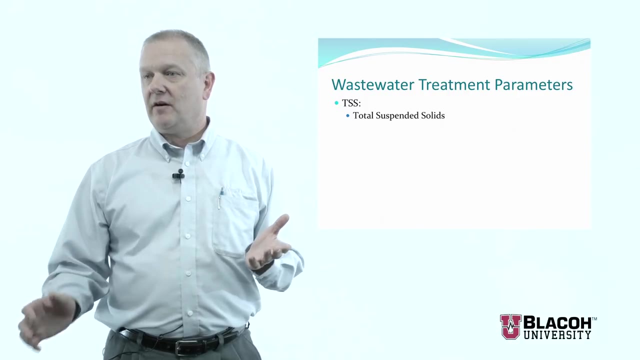 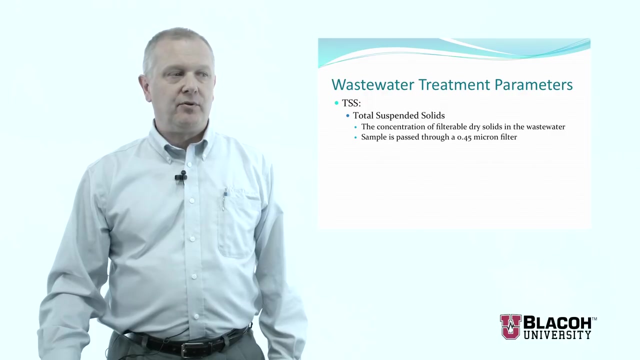 in milligrams per liter or parts per million. So it's very effective process and it does a good job. Let's move on to TSS, or total suspended solids. This is a measure of the particulate matter in the wastewater. What we do is we run the wastewater sample through. 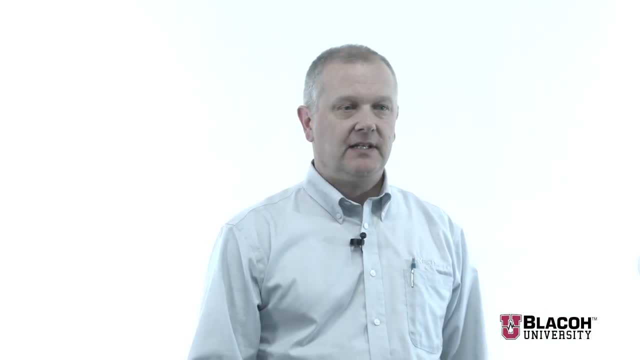 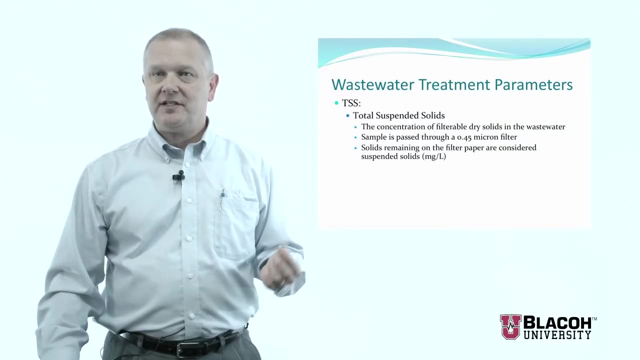 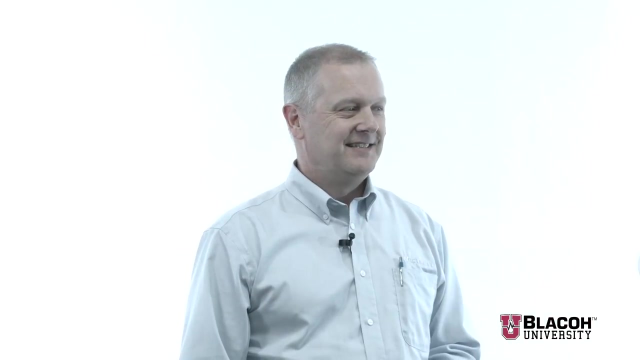 a 0.45 micron filter Uh procedure And whatever stays on the filter paper is considered suspended solids. Obviously there are some very refined solids that do go through, but we consider those dissolved because they are so small that essentially they are You dry that the solids on that. 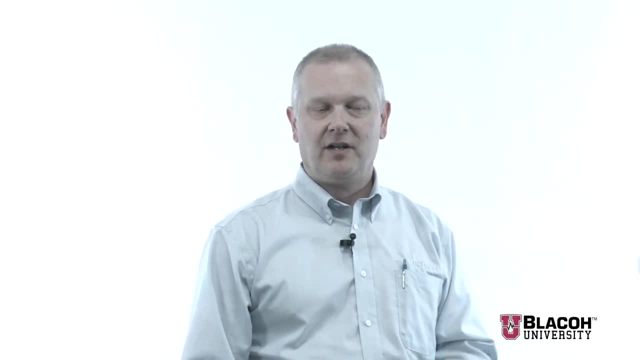 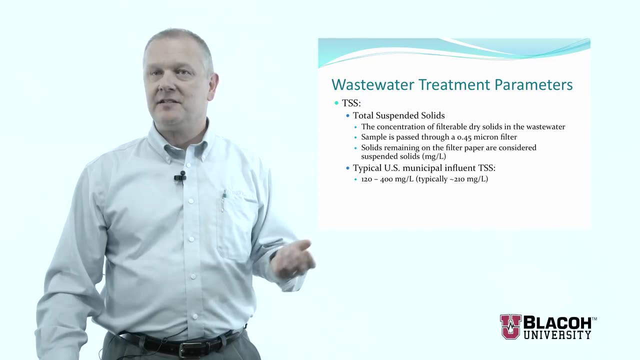 filter paper. weigh it. now you have the suspended solids concentration for that wastewater And again, the typical influence coming into a sewer treatment plant in the United States is somewhere around 200 milligrams per liter. There's a range there again, depending. 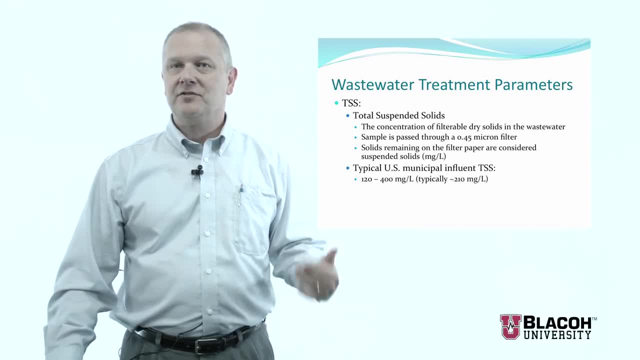 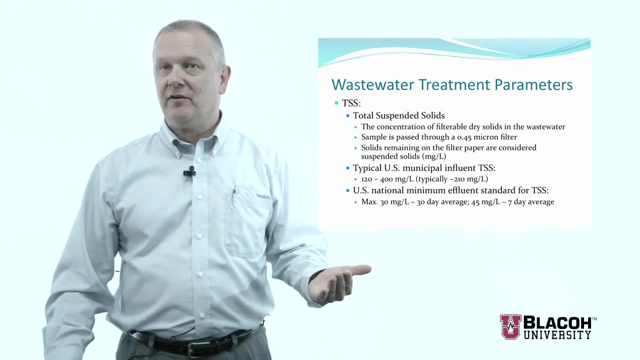 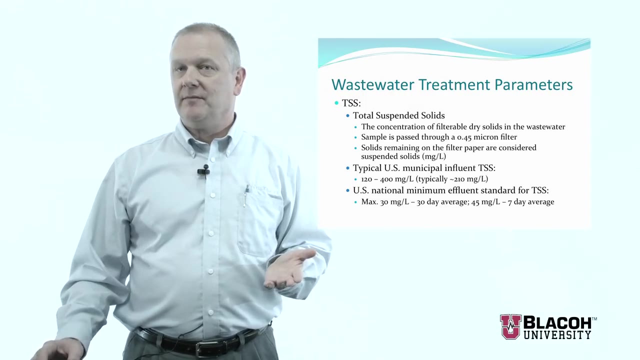 on the type of community and the industries and so on that are in the community. Again, the US national minimum standard is 30 milligrams per liter of suspended solids going out of the treatment plant in a 30-day average Over seven days. 45 milligrams per liter, And again. 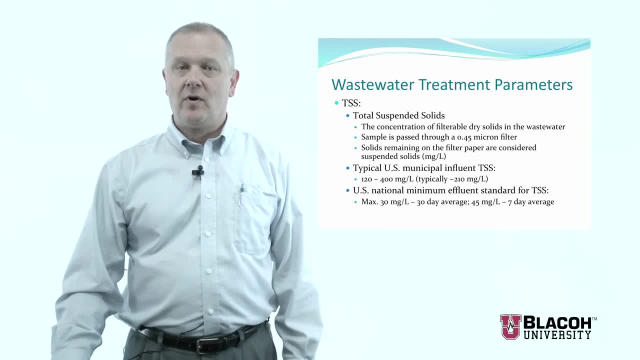 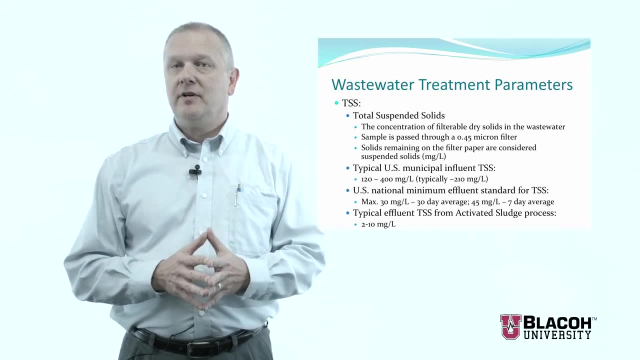 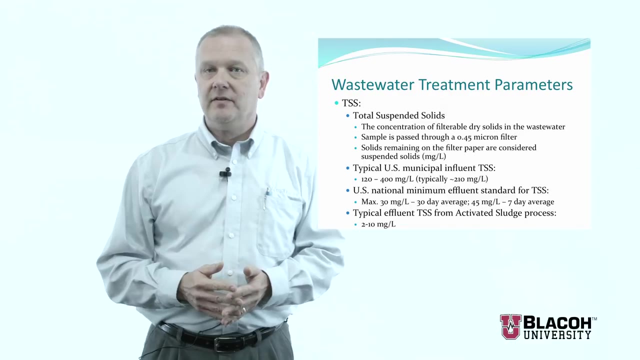 much tighter in certain areas of the country, depending on the water body that it's going into. Typical TSS coming out of a treatment plant that's using an activated sludge process is in the single digits. So, again, very effective in removing the particulate matter from the 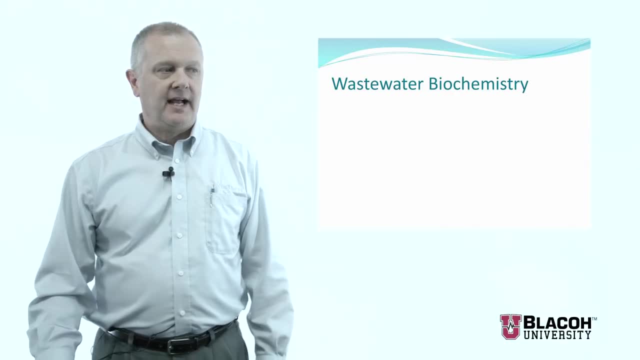 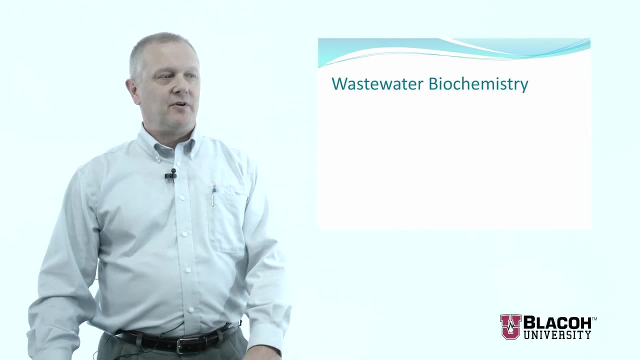 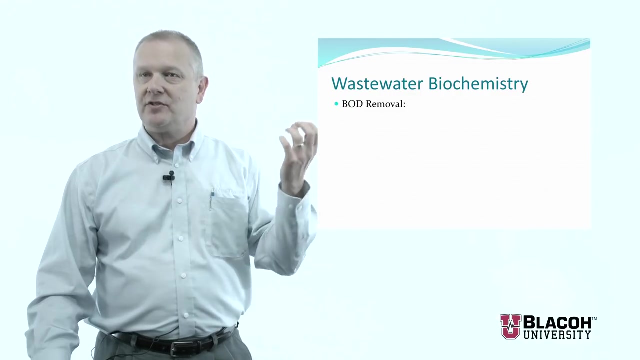 waste stream. Okay, let's look at very briefly some biochemistry, And this is not very technical, but basically we want to talk about what goes on and what the microorganisms do as they remove this BOD or this organic matter from the wastewater When there is oxygen present. 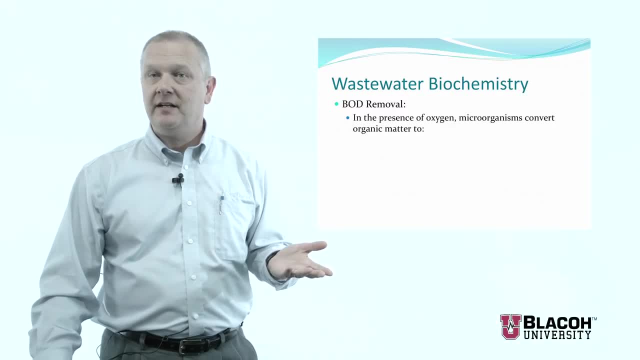 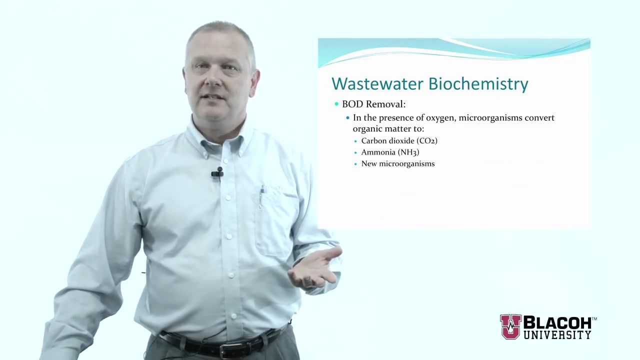 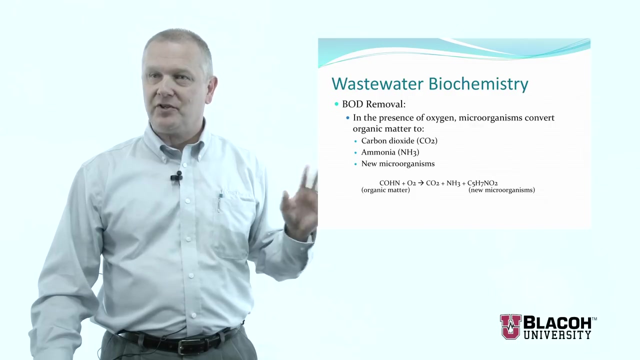 the microorganisms convert this organic material to carbon dioxide, ammonia and new microorganisms. Obviously, they're reproducing and growing. Those substances are fairly harmless. Now ammonia has some problems, and we'll talk about ammonia later- But this is the way. 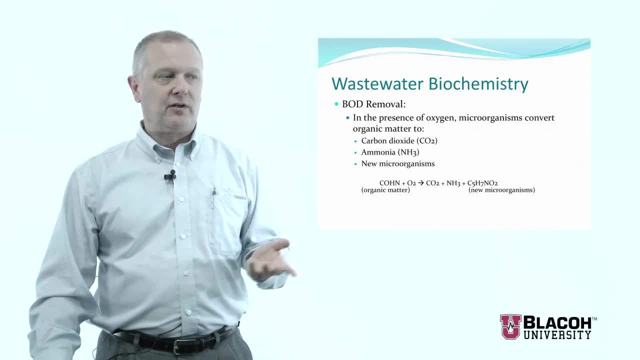 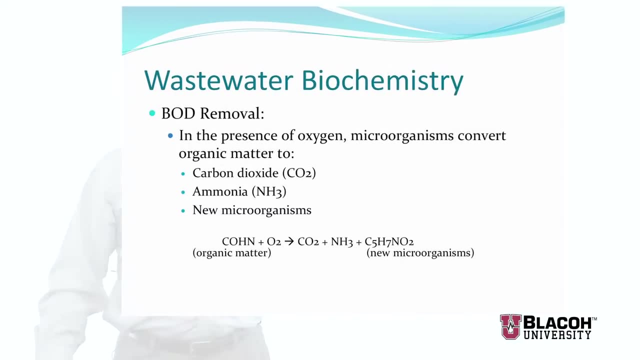 way. this is the basic process that goes on. now, if you try to write a chemical equation, this is not a balanced chemical equation because there's all kinds of different organic chemicals that you'd have to to include in that. but basically on the left side of the equation we have COHN, meaning some type of organic. 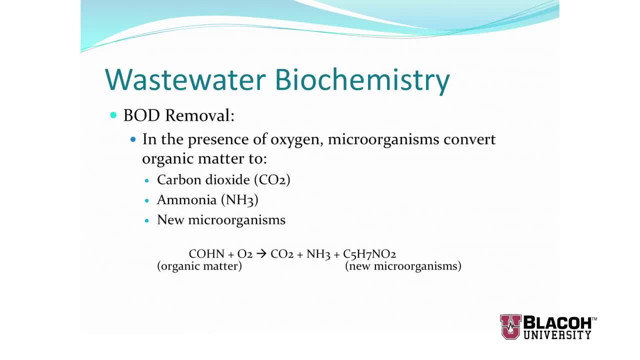 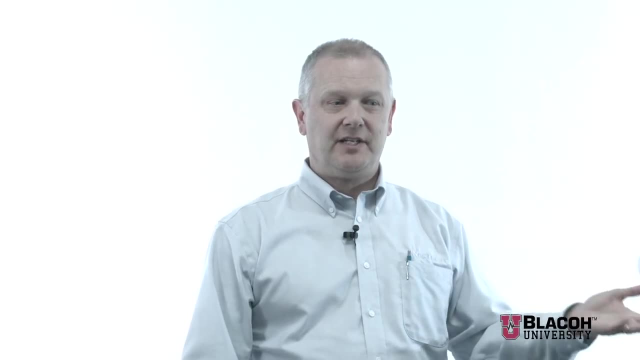 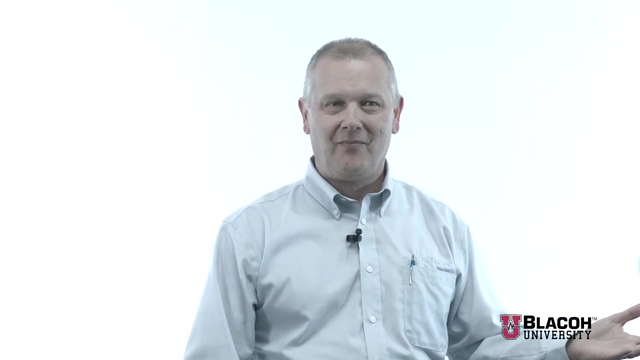 chemicals combined with oxygen in the presence of microorganisms. you get from that CO2, ammonia, and that's an approximate chemical formula for bacteria, new microorganisms. now, I said, this was the equation, the biochemical equation for removing BOD. where's the BOD in this equation? well, remember BOD. 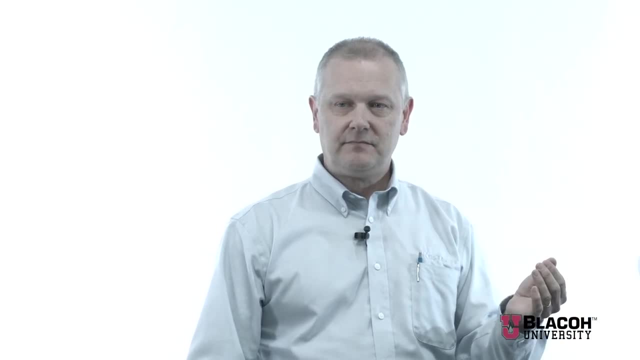 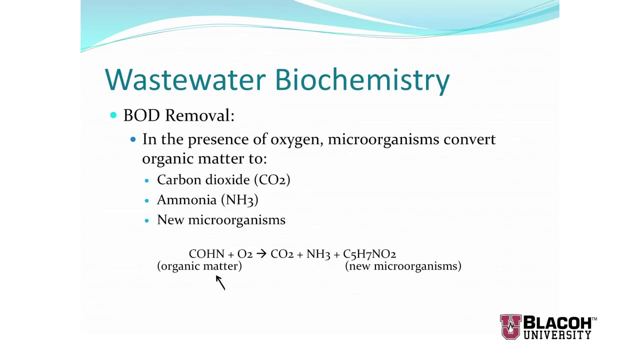 stands for biochemical oxygen demand, meaning it's the oxygen that's absorbed in the biodegradation of the BOD of this organic matter. So in a sense it represents the organic matter. It's a surrogate for actually trying to measure all of these different organic chemicals and their concentrations. 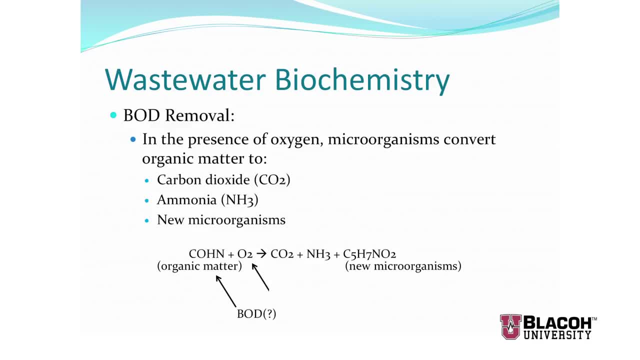 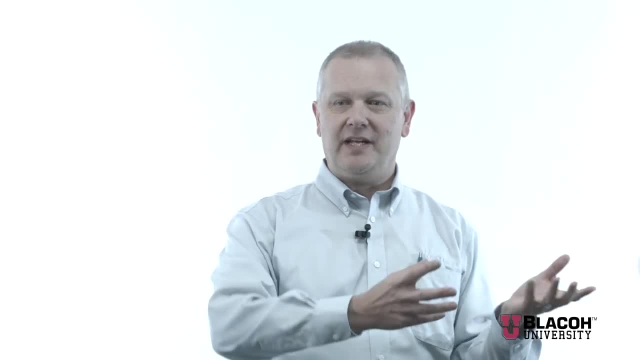 You could also say: well, it is the oxygen that's being consumed by that. In the wastewater industry they're kind of used simultaneously And we often talk about removing BOD as if BOD were a substance. It's really a surrogate for all of this organic matter, the urine. 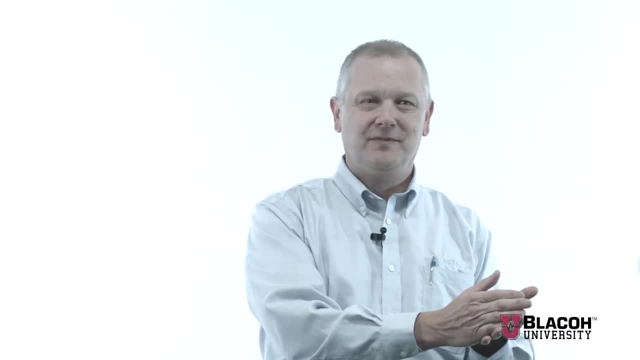 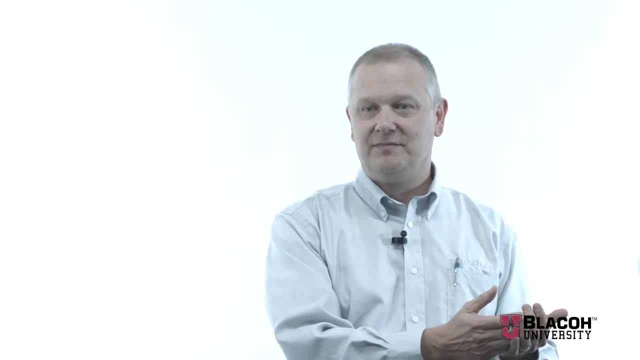 the feces, the food products that are ground up in your disposal and everything else that ends up in the sewer that's organic in nature and can be degraded by these microorganisms. So when we talk about removing BOD, or how much BOD is in the wastewater, a lot of times 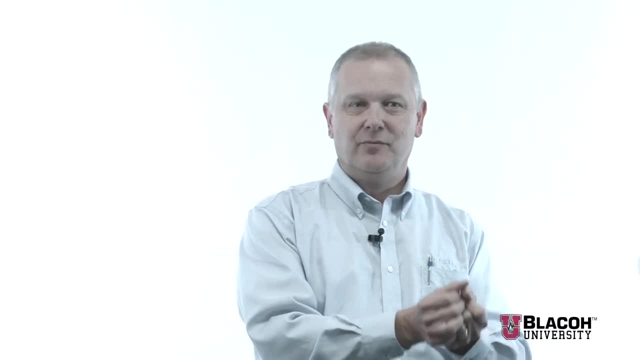 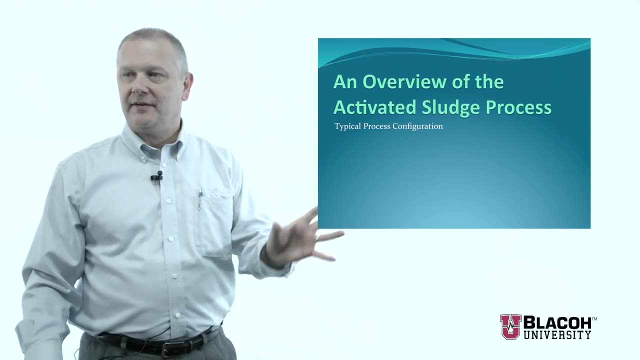 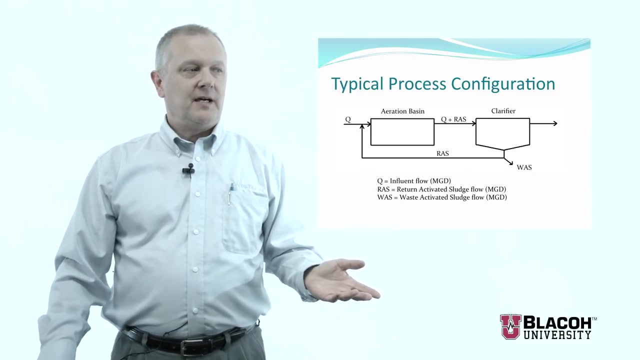 the professionals are really meaning: how much organic material is there that we need to get rid of? All right, let's talk about a typical activated sludge system and what that looks like. Okay, This is just a very simple diagram. Basically, we have a large tank we call an aeration basin. 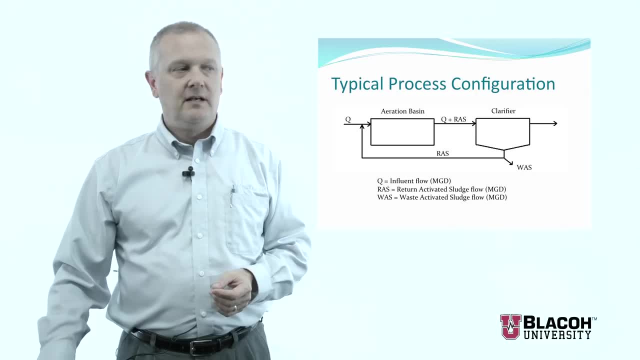 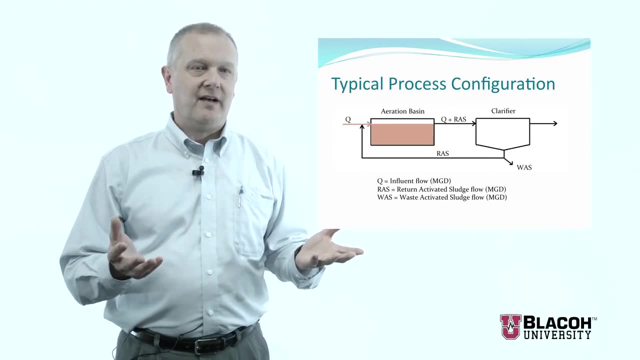 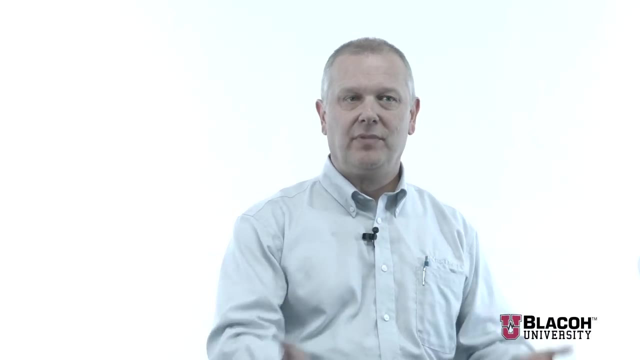 and we have a clarifier, which is a settling basin. Our flow comes in to the aeration basin, fills that up. Now, in an aeration basin we have, logically, some kind of aeration system. We either have diffusers on the floor that bubble air up through the liquid or we have some kind. 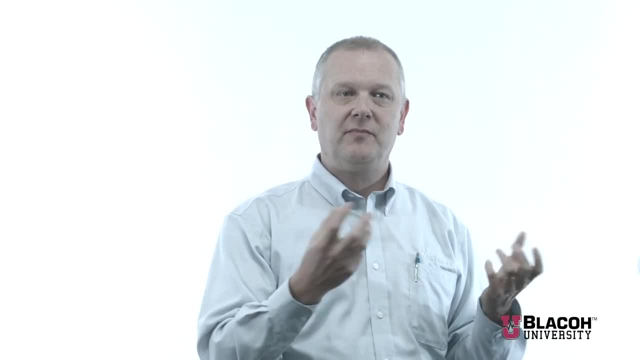 of mechanical system that's going to be able to move the air up through the liquid. And we have some kind of mechanical system that's going to be able to move the air up through the liquid. And we have some kind of mechanical device that stirs and churns up the liquid and gets 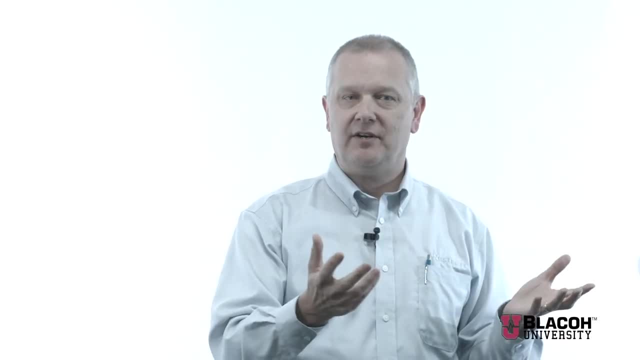 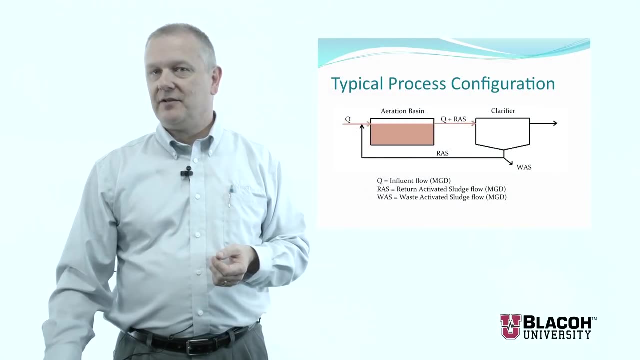 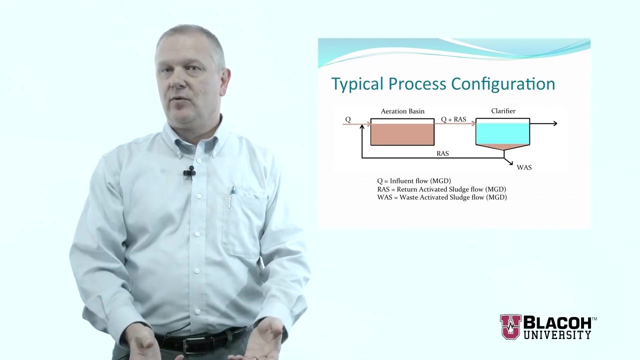 oxygen and air to dissolve in that water so that there's plenty of oxygen for the microorganisms to do their job. From that point the liquid goes into the settling basin or clarifier, and the microorganisms actually settle to the floor of the clarifier And the liquid that comes out. the top is 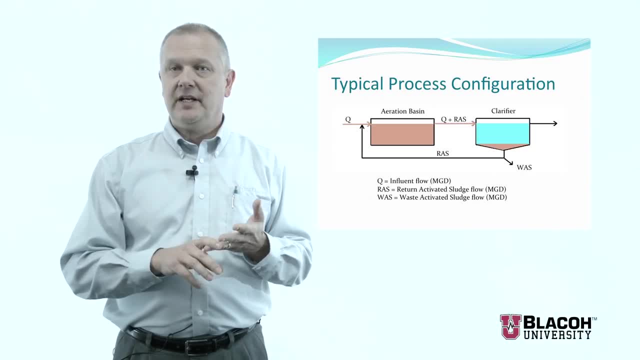 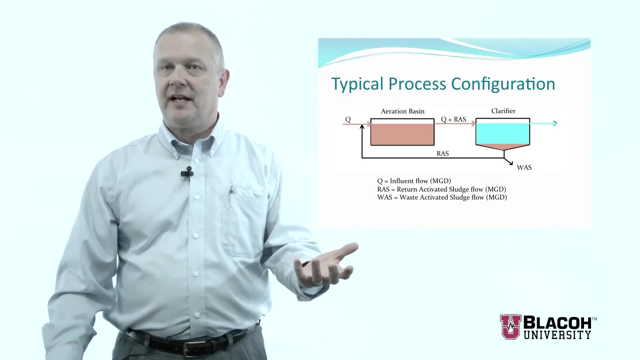 like I said, typically single digit in volume, BOD and suspended solids, And so the clear liquid flows out the top, but we take the solids that settle in the bottom of that clarifier and we recycle them. We call it return activated sludge. 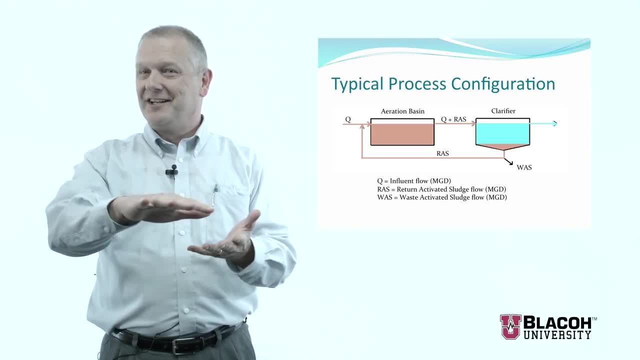 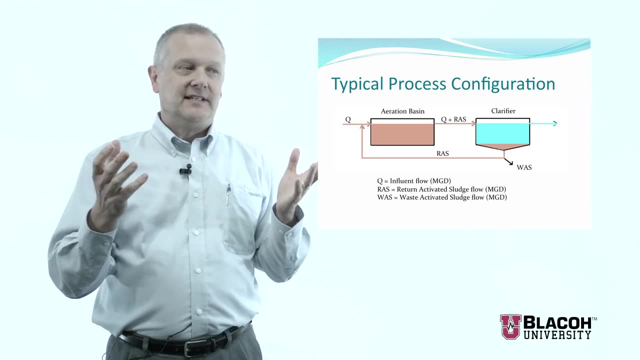 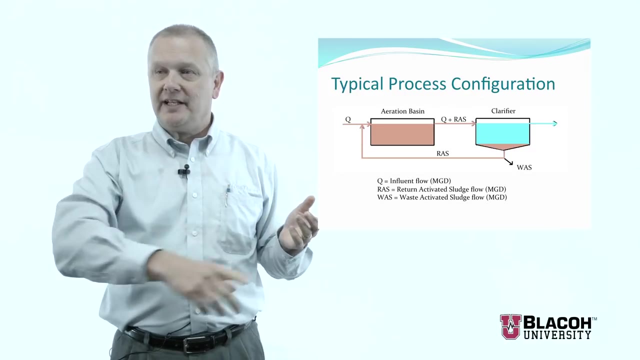 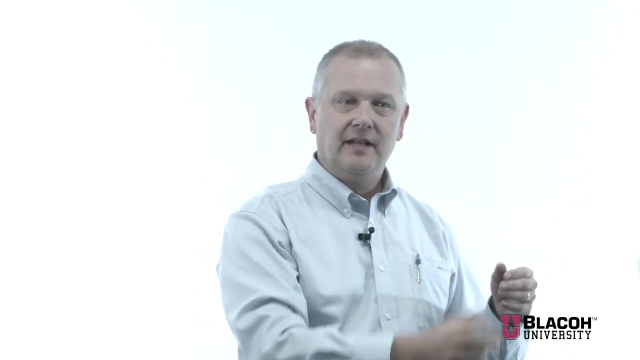 into the aeration basin. So the sludge that settles in the clarifier is recycled into the aeration basin and activated to work on the contaminants that come into the system. So the when we keep doing that until we have maybe 30 times the amount of microorganisms in the system. 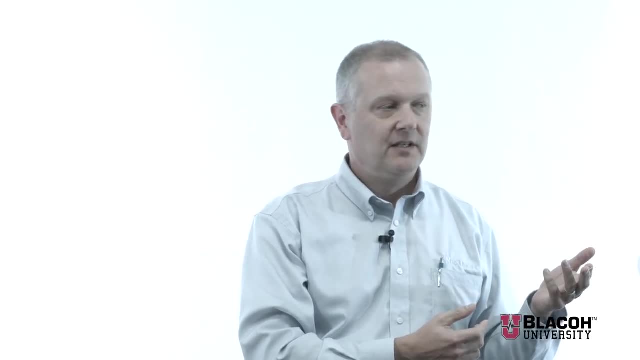 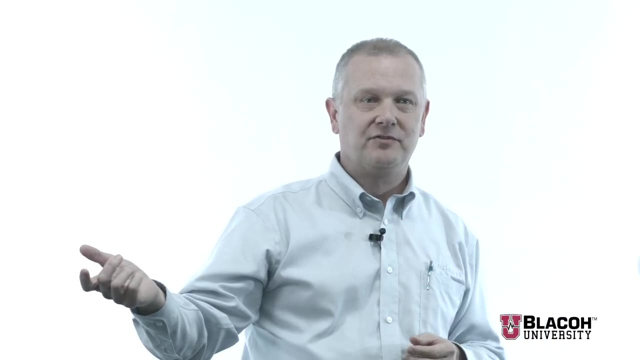 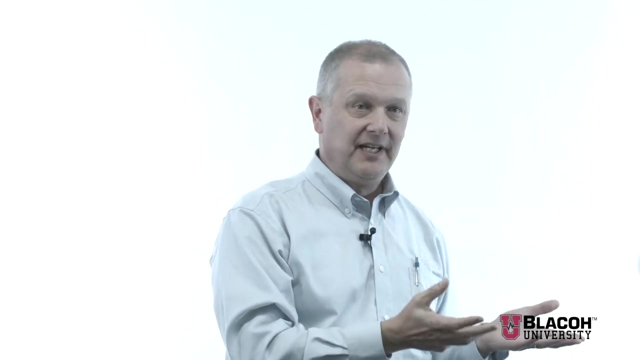 than we had in the waste stream that was coming into the plant in the first place. So we can degrade this organic matter 30 times faster than if you were to put it in a stream. That's the whole. goal is to use the natural biological forces in nature to clean the water, but do 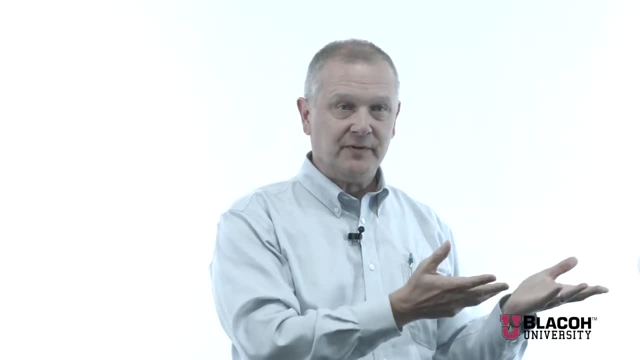 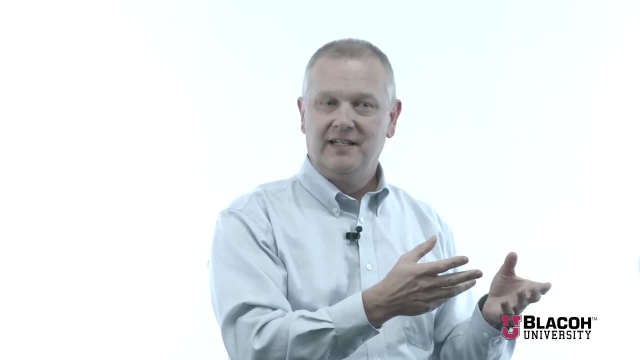 it quickly and in a confined space, And that's the reason we use the sludge. The reason we have to add the air to the tank is because, with that many microorganisms, they're using a lot of oxygen and we have to add extra oxygen rather than just what. 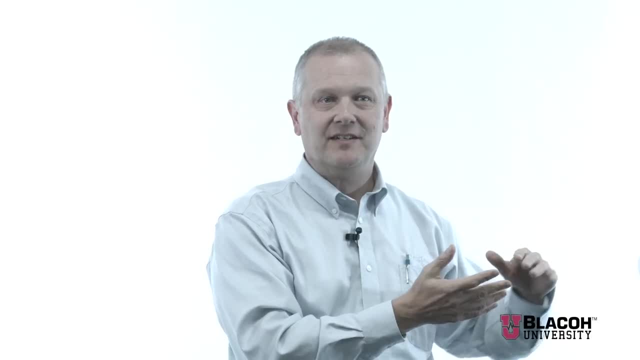 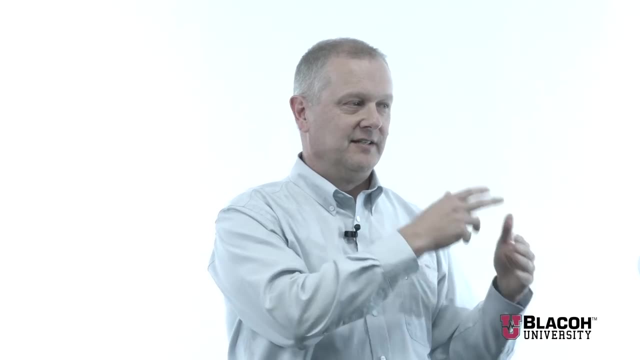 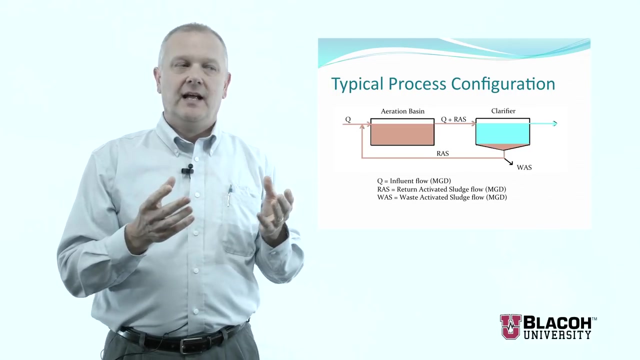 is going to dissolve in the water, through the atmosphere, And so we have to provide that extra aeration. Now, this is not just a mass balance of solids in and solids out, because these microorganisms are growing and multiplying, And so there's significant amounts. 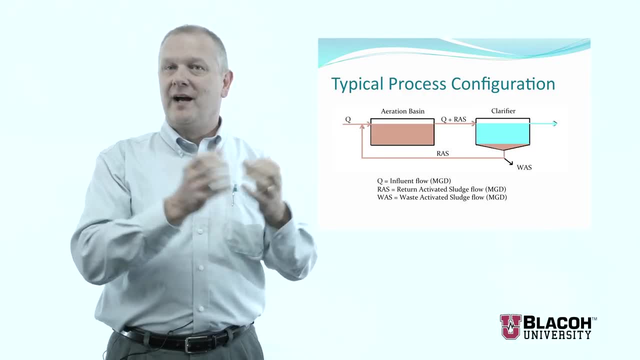 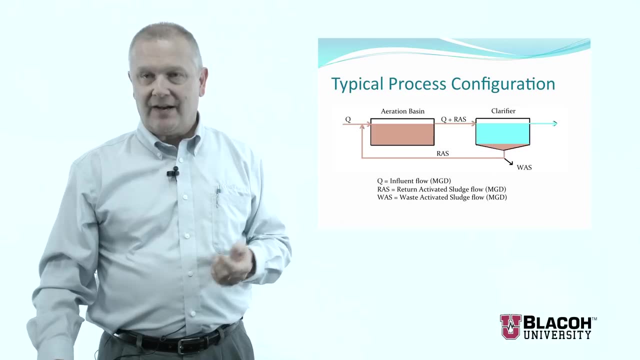 that are actually generated by this process. It's new microorganisms that are growing. They're absorbing this organic matter and growing new cells, So you have to remove some from the system. That's what we call WAS or waste-activated sludge- the solids that are 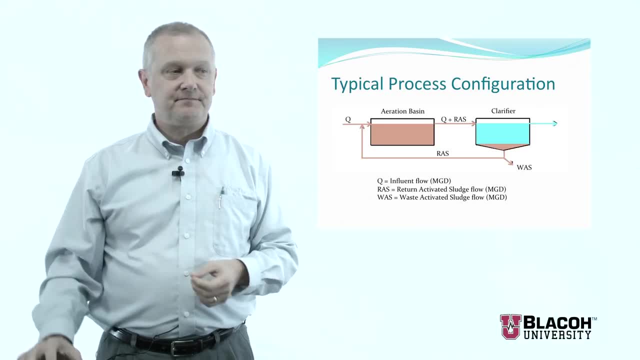 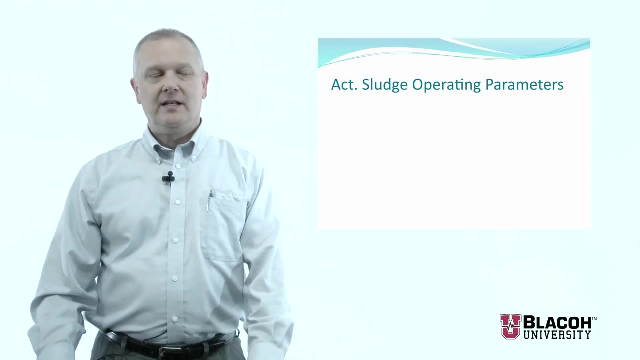 wasted from the system and disposed of. Let's talk about some operating parameters in activated sludge. These are not terribly difficult systems to operate, but there's some important things that need to be watched so that the system performs properly. The first one we'll talk about is the mixed liquor. suspended solids concentration- Mixed. 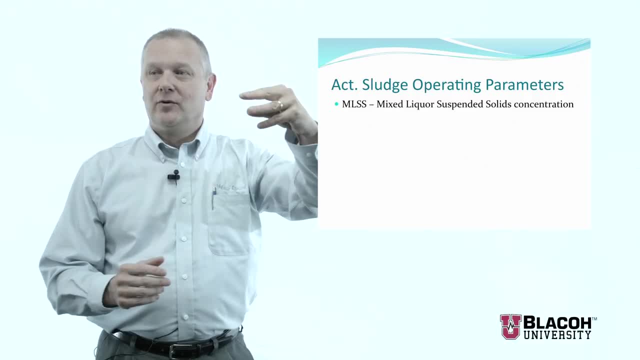 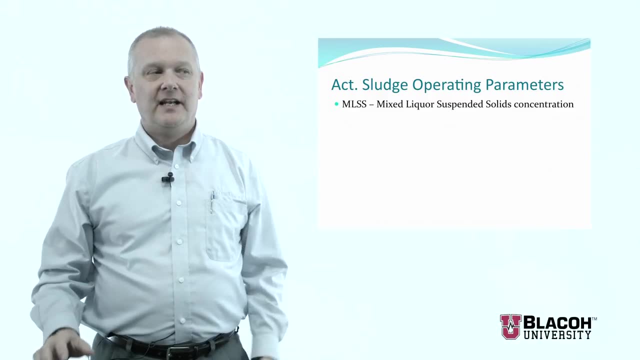 liquor is called that because it's a mixture of the raw feed coming in and the returned sludge from the clarifier. So it's mixed to form this liquor and it has a concentration of solids. Typically we'd use it to form a good level of drinking water, but it's a 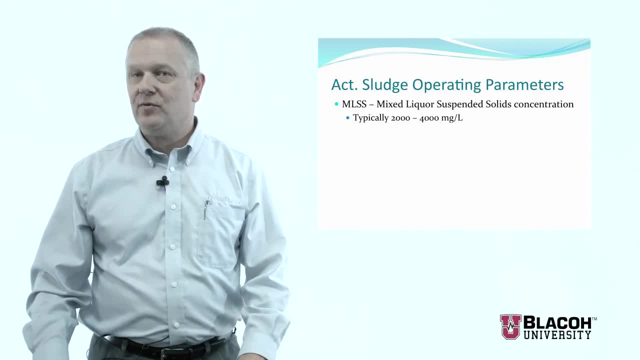 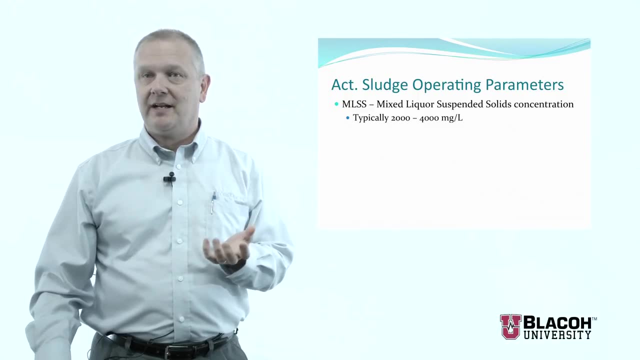 Typically in an activated sludge system, that's anywhere from 2,000 to 4,000 milligrams per liter of solids, most of which is actually the bacteria that are doing the work to break down the organic material in the waste. If you can run at a higher mixed liquor concentration, you don't need as big a volume because you can pack them in tighter and treat in a smaller footprint. But the maximum concentration you can practically get by with is limited by a couple of things. Air requirements, that is, if you pack them in too tight, you cannot physically get enough air dissolved in the water to keep all the bugs alive and active. The second problem is in your settling basin. If you have too high a concentration of solids it will not settle as rapidly. 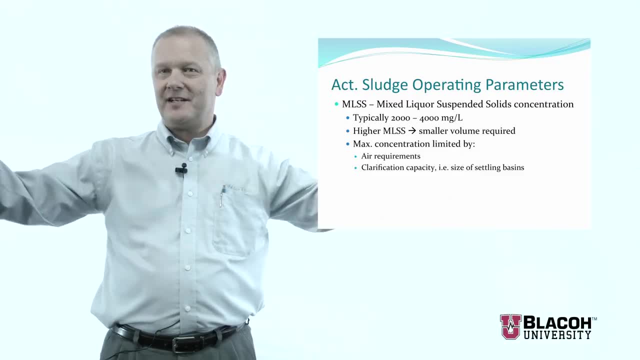 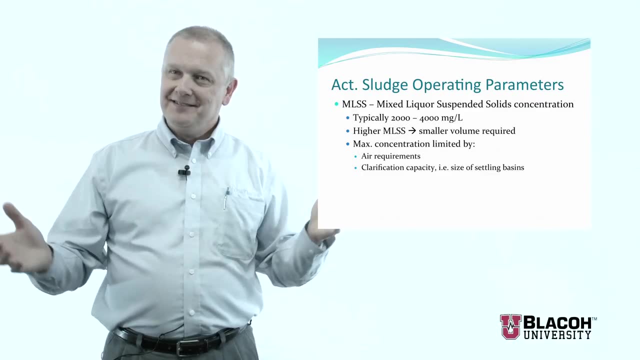 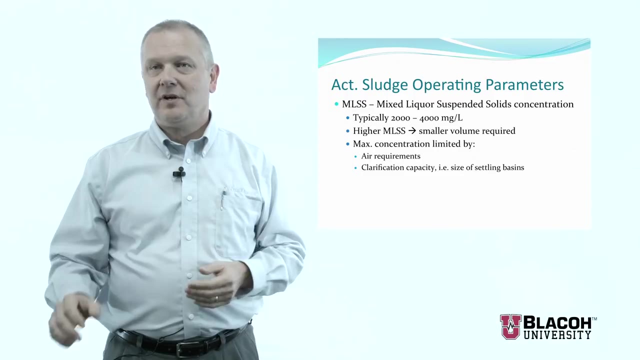 And you'll need immense clarifiers to try and settle a very, very thick or very, very high concentrated solids, And so that limits the concentration that you can build this aeration basin concentration up to- And, like I said, typically it's between 2,000 and 4,000 milligrams per liter. 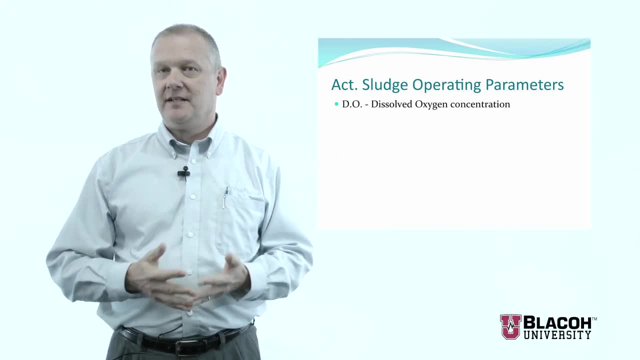 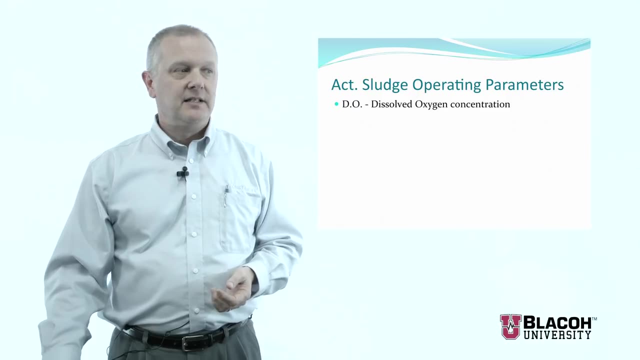 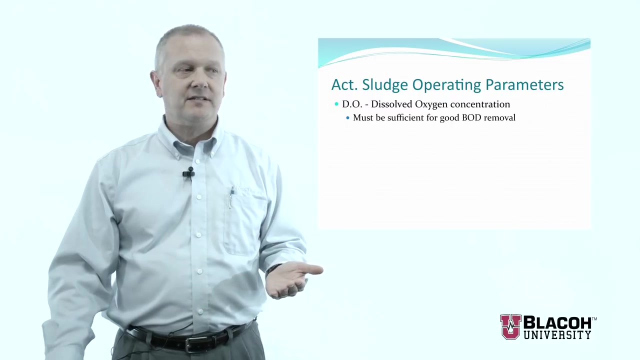 Dissolved oxygen concentration. This is obviously critical, As I've talked about. these microorganisms respire and they need to be dissolved. They need the oxygen dissolved in the water to work correctly. It has to be sufficient to really degrade all the organic matter or BOD in the waste. 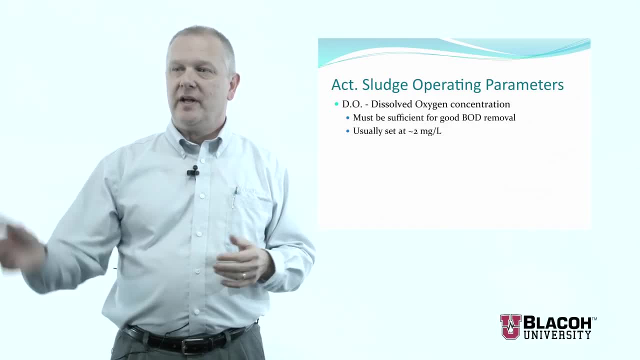 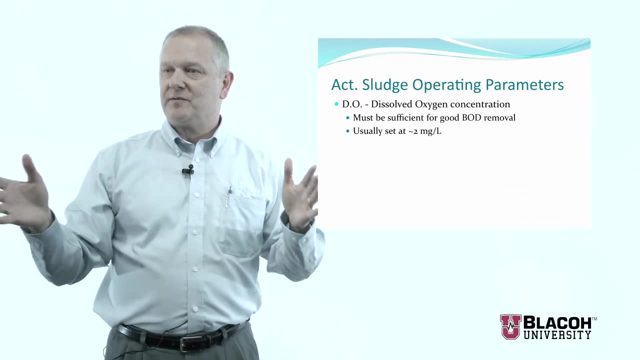 Usually we set it at about 2 milligrams per liter. So we have an oxygen sensor in the aeration basin at all times and we keep the level in that basin at about 2 milligrams per liter. So there's a little bit excess oxygen that's always there for the microorganisms to do their work. 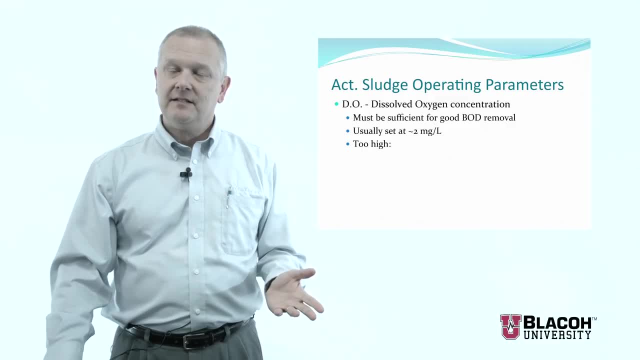 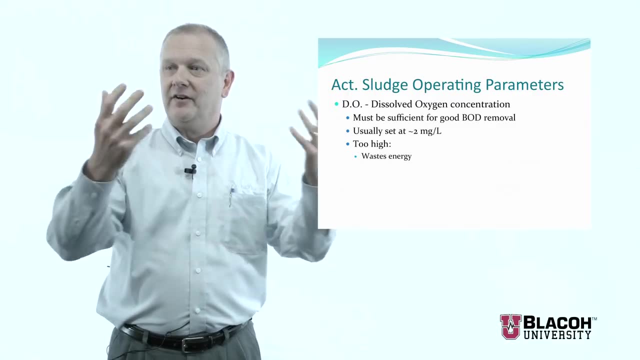 If you set it too high, there's a couple problems. First of all, it wastes energy. You're spending a lot of energy churning up the liquid or blowing air into the liquid, And that's a very expensive. part of the waste treatment process is this aeration. 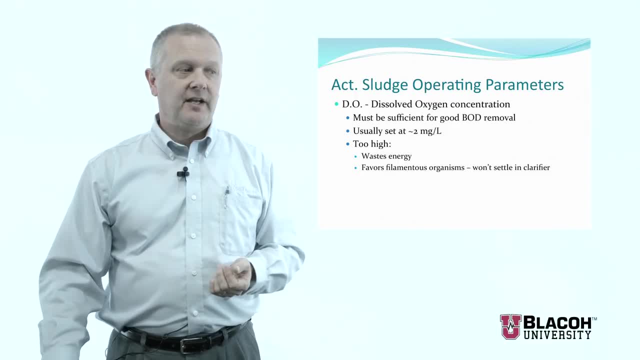 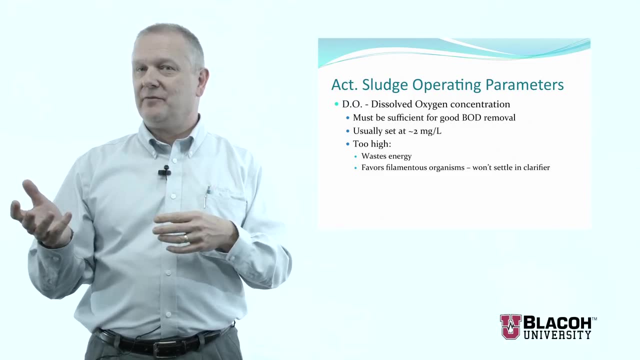 And so you don't want to set it too high. On the other hand, oh, and also if it's too high, you create an environment that favors a certain type of bacteria that we call filamentous bacteria. Most of the time, it's not filamentous. 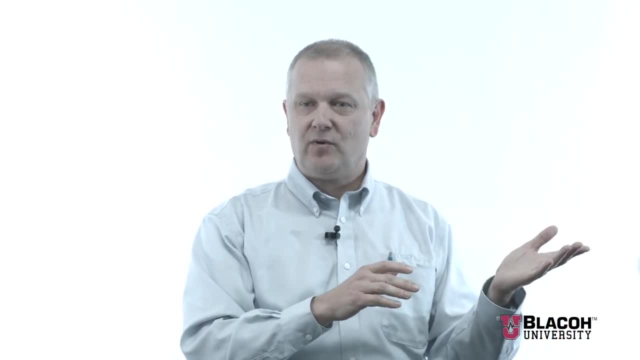 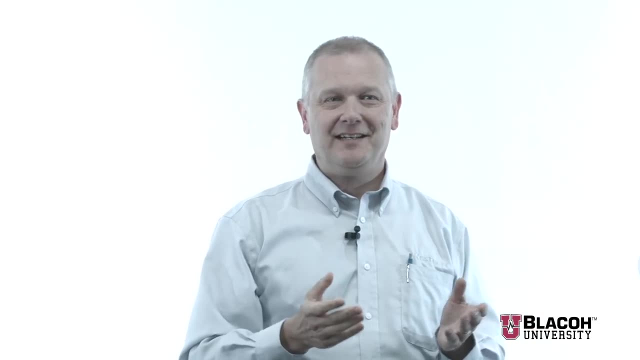 Most of the time it's not filamentous. Most of the time it's not filamentous. Most of the bacteria that do this BOD removal for us are small, round or oval-shaped bacteria like you see in your lab microscope if you've taken any biology classes or anything like that. But there are other types of bacteria that are filamentous. They look like tree branches or feathers with long filaments. They like the environment with a lot of oxygen, And so we'll grow more of those if we have too much oxygen in the system and they don't. 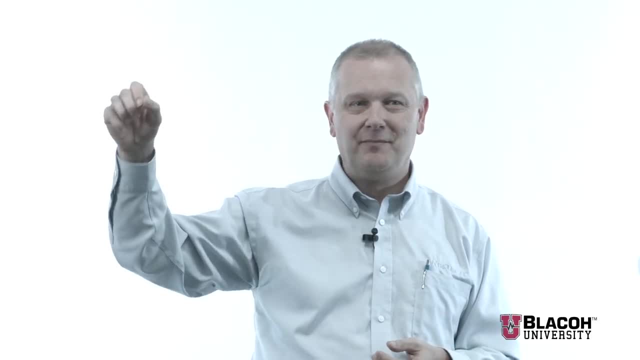 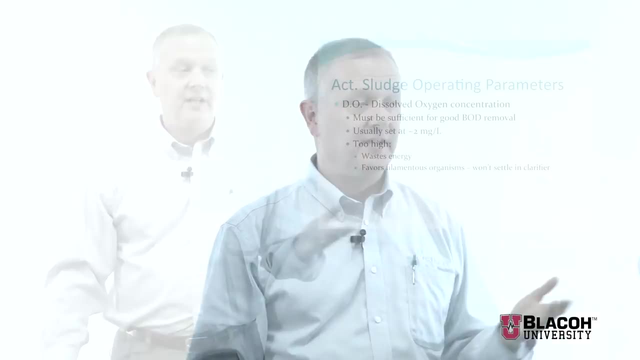 settle well in the clarifier. It's like dropping a feather: It doesn't drop nearly as fast as a rock. Very similar analogy. So we don't want the oxygen too high in the system. On the other hand, we don't want it too low either. 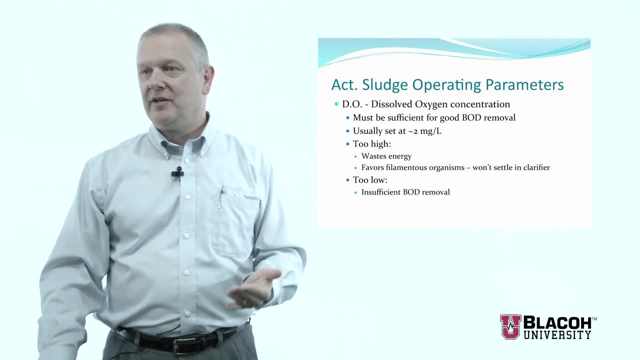 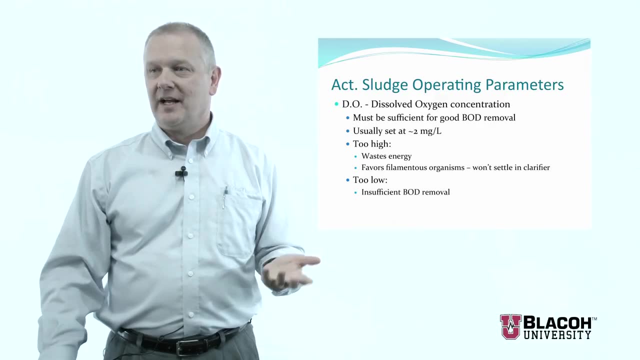 If it's too low, you're not going to get the BOD removal you need, because the bugs- we call them bugs- the microorganisms- can't remove the organic material And if it gets really low it will go anaerobic. 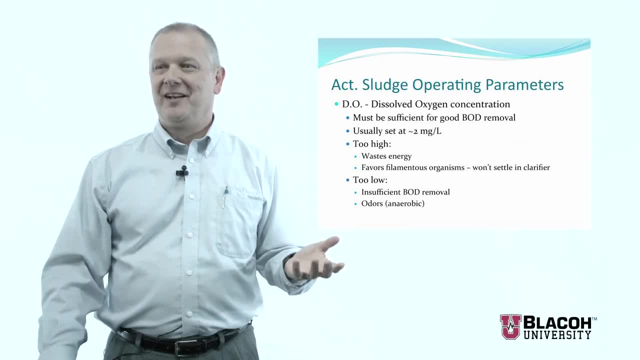 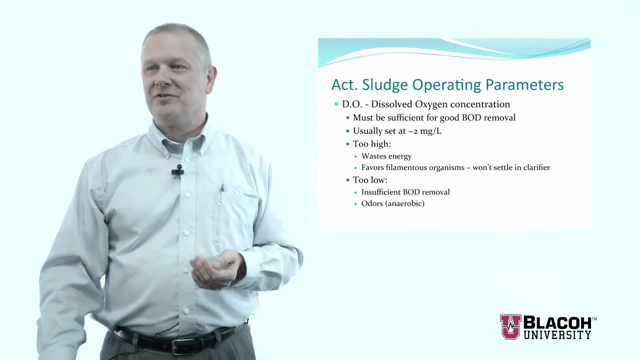 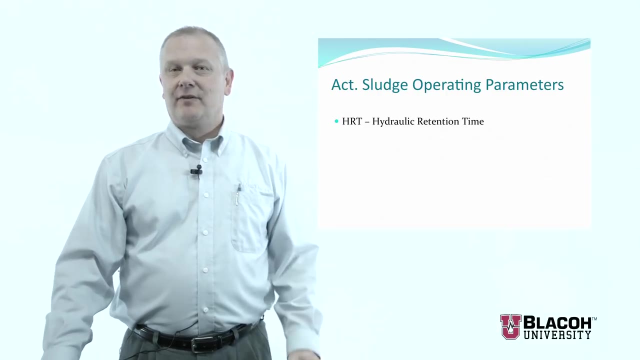 Which to most of us means it's smelly, It's gone, rotten and it stinks. You're going to get hydrogen sulfide and other gases that the neighbors around the treatment plant are not going to appreciate. Hydraulic retention time is the time the liquid stays in the system. 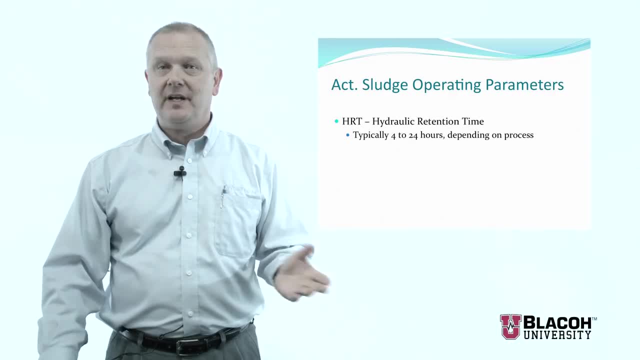 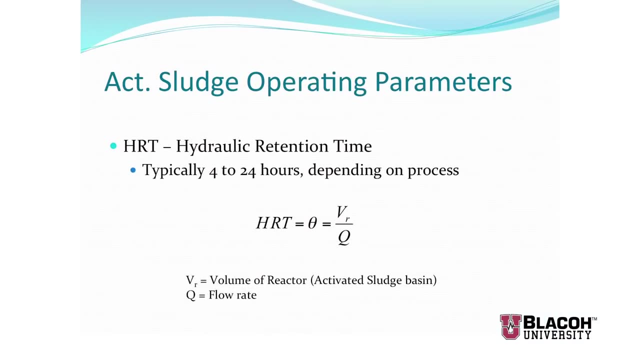 Pretty straightforward: Typically four hours to 24 hours, depending on the process and how much contaminants we need to remove. Okay, Simple equation: The hydraulic retention time is the volume of the reactor or the aeration basin divided by the flow rate Q, And that gives us an average time that the liquid is in the system. 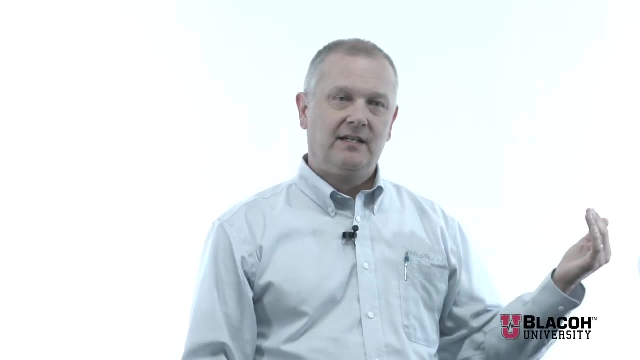 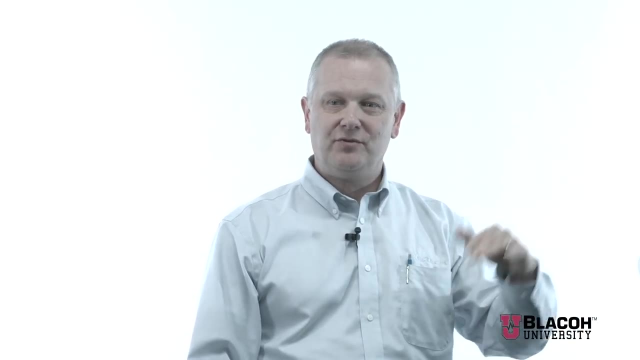 That's a simple parameter, but it's important. If you have, say, you have a storm and your city is one of those unlucky cities that has combined sewers, that means the storm sewers and the sanitary sewers go to the same pipes. You have a big storm, You suddenly get a great increase of flow through your treatment plant And if that hydraulic retention time is not long enough, it's not long enough for the bugs to eat the organic material that's in the water. So you do have to watch that and size the basin so that you have enough retention time. 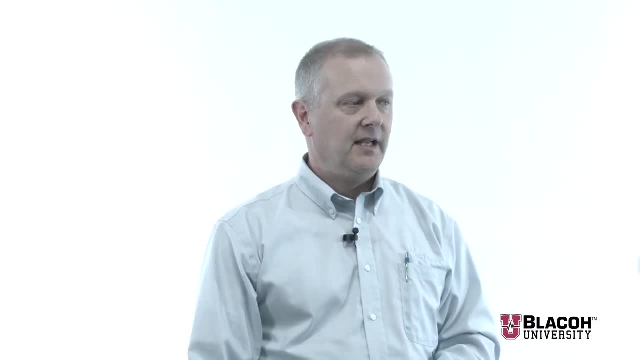 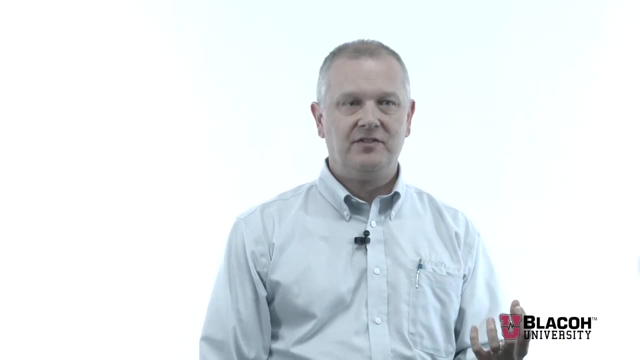 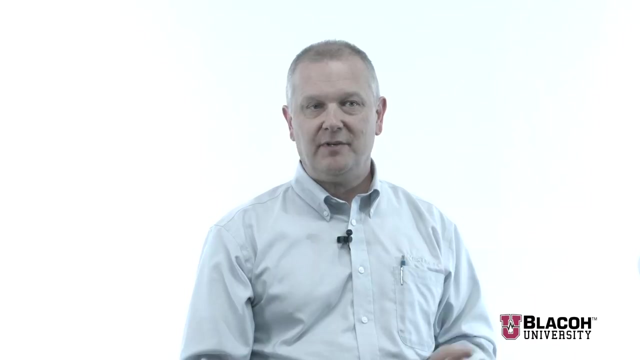 for the microorganisms to do their job. Even more important in this type of a system, though, is the solids retention time. How long do these microorganisms stay in the system? Okay, Recycling them back from the clarifier over and over again. the solids retention time. 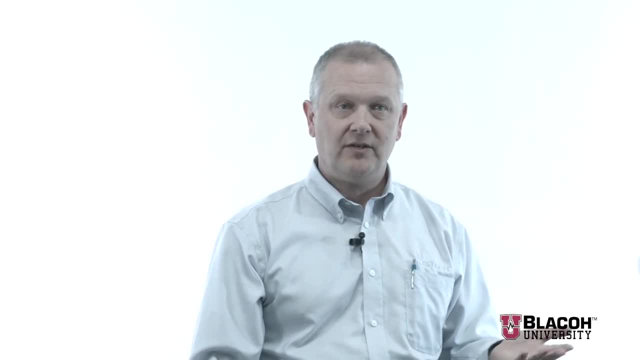 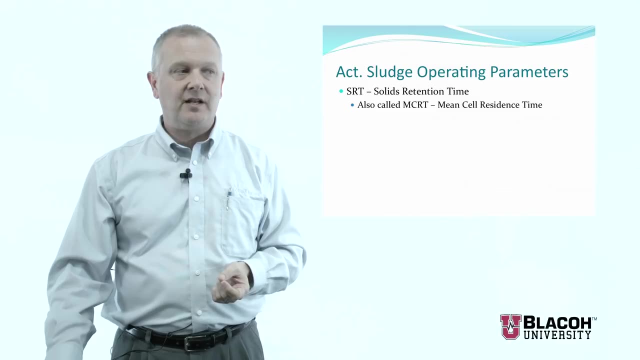 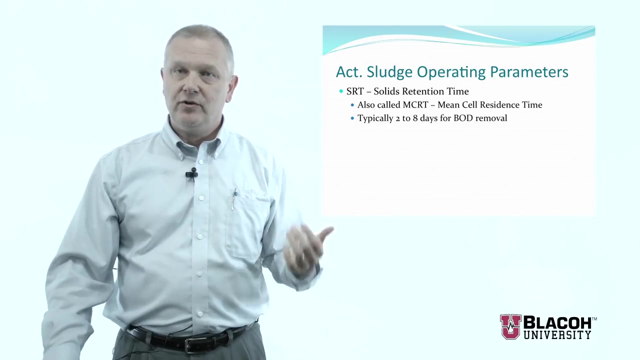 is much longer than the liquid or the hydraulic retention time. We also call this the mean cell residence time, because these are bacterial cells that we're talking about. Typically it's two to eight days for simple BOD removal. If we get into nutrient removal processes, which is another class that we'll talk about, it's even longer, But for typical BOD removal most wastewater plants, this solids retention time is between two and eight days, And it needs to be long enough that we allow the organisms to reproduce and grow. If our SRT is shorter than the reproductive cycle of the microorganisms, they'll be. 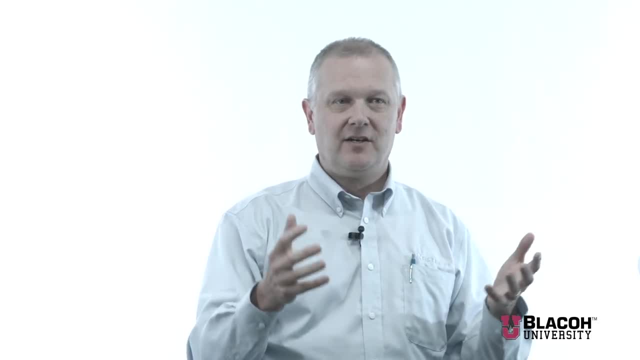 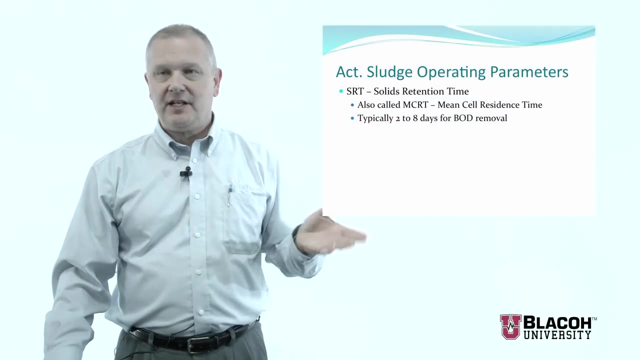 out of the system before they reproduce and we can't get the concentration we need to do the job. So this is a very important parameter that we have to design, for This is the equation. It's a little complicated, but it looks a little complicated, but it really isn't. 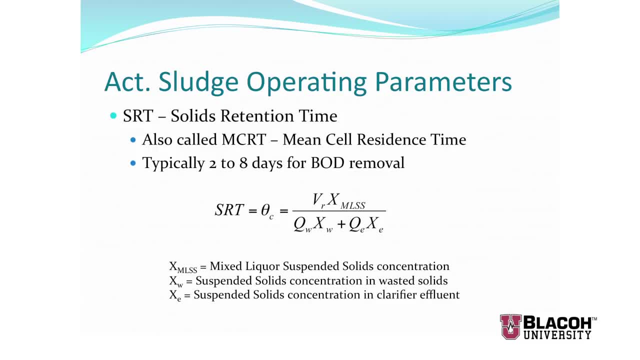 The SRT is basically just the volume of the reactor times the concentration of solids in the reactor, which gives you a mass of solids divided by two things. We have the waste sludge that's leaving the system that's represented by the Q sub W. 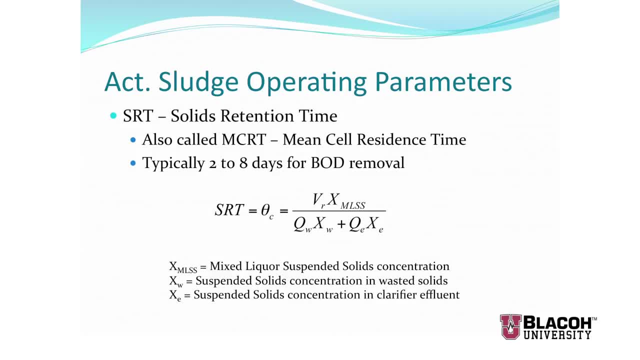 times the X sub W, X being the concentration in those wasted solids, Q being the flow rate of the wasted solids and the solids leaving the system in the effluent of the clarifier, which we hope is very small. But to be technically correct we have to include it in the equation. 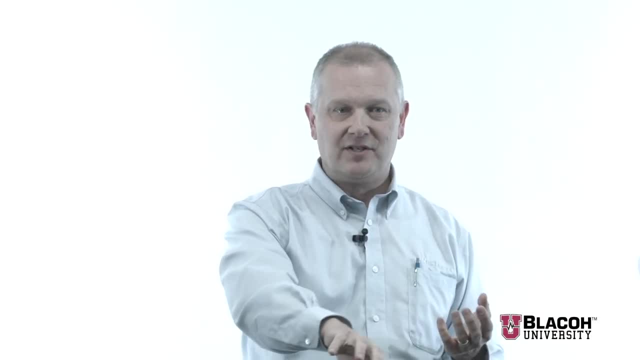 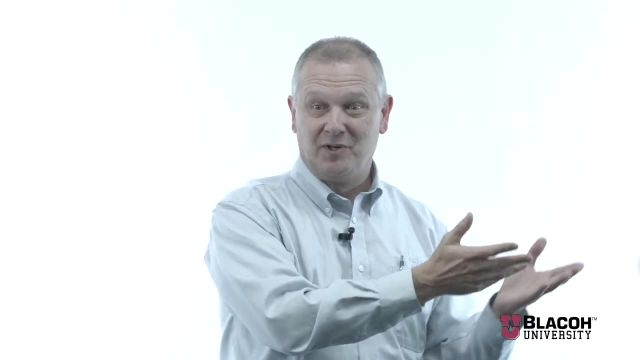 In practical circumstances. a lot of plants don't even use the effluent solids in this equation when they calculate their SRT, because it's pretty negligible compared to 2,000 milligrams per liter in the aeration basin And you may be getting five. 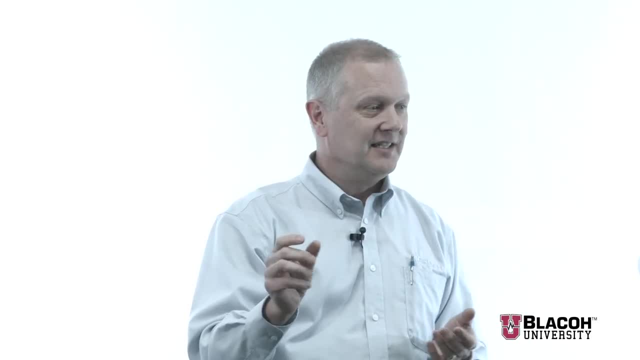 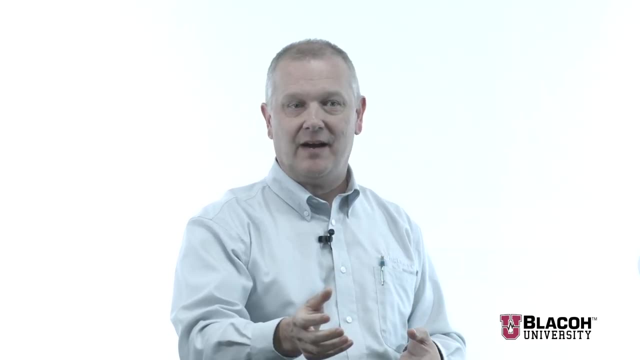 I don't know, Five out of the clarifier, not 5,000, five, And so all we're doing is we're saying here's the total mass of solids and here's the amount that's going out. So that's what this equation represents. 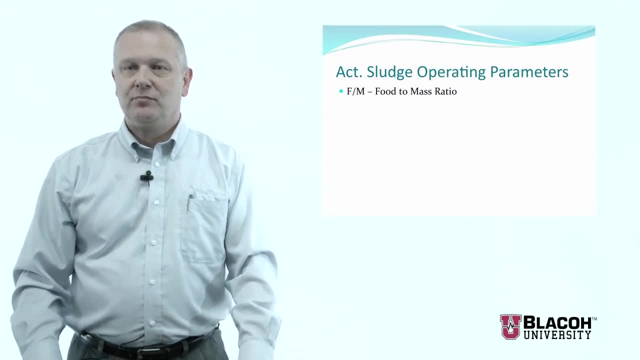 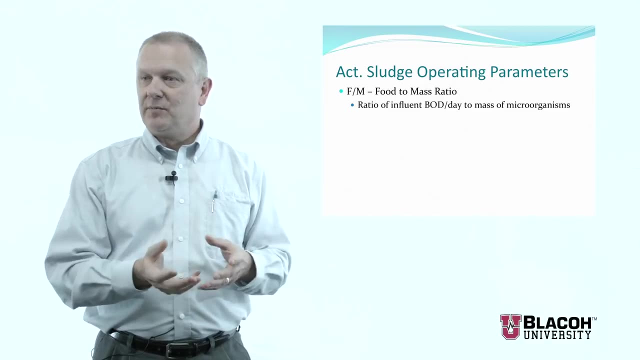 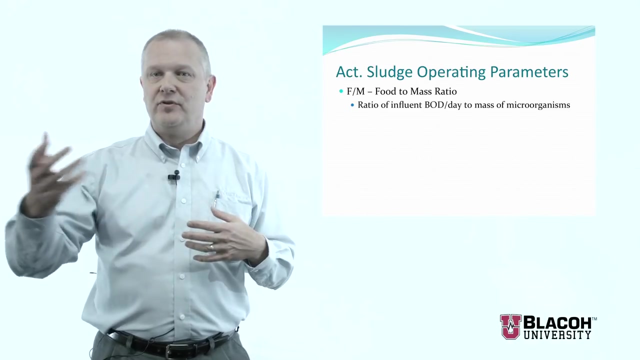 Finally, another parameter that's important is what we call the food to mass ratio. This is a ratio of the BOD coming into the plant per day to the mass of microorganisms that's there. You can liken this to the amount of food that you eat every day divided by your weight. 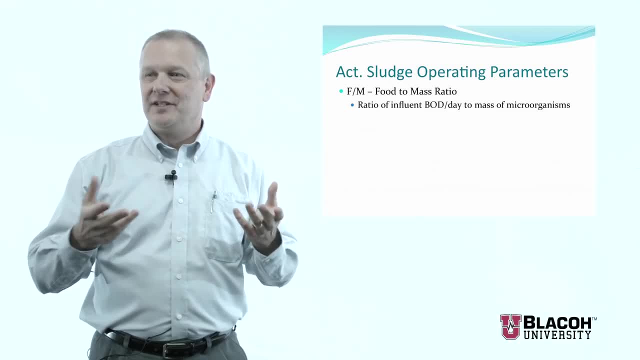 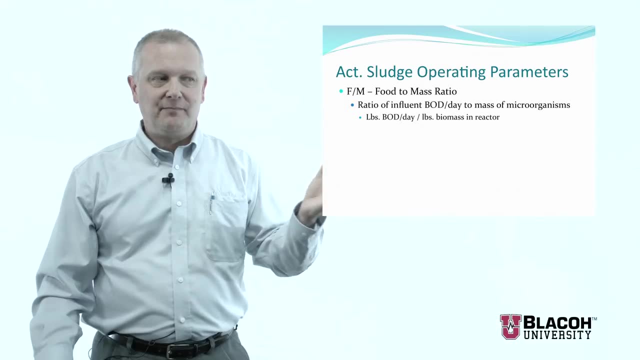 Somebody who weighs 200 pounds can eat more in the way of calories and food than somebody who weighs 100 pounds. Same is true in microorganisms. This is measured in pounds of BOD per day divided by pounds of biomass or solids in the reactor. Normal range is 0.2 to 0.5.. You or I couldn't eat 20% to 50% of our body weight. We could eat 50% of our body weight. We could eat 50% of our body weight. 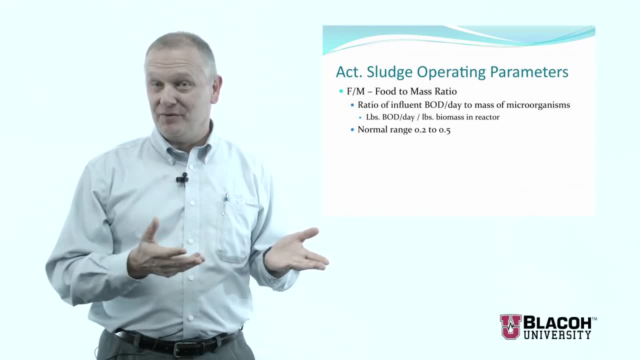 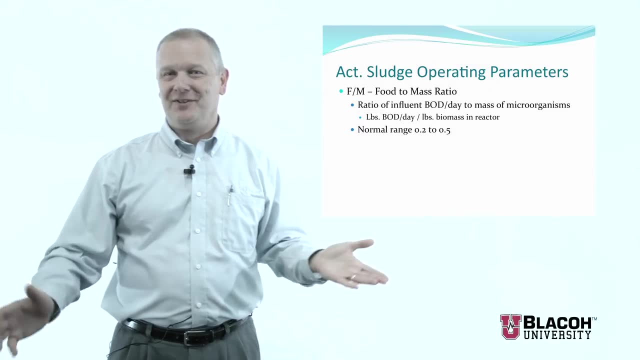 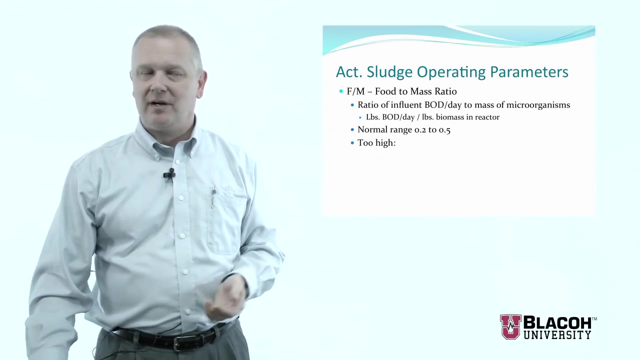 We could eat 50% of our body weight in food every day, But microorganisms do. They have much higher metabolisms than you or I do, which is lucky, because otherwise we'd be drowning in waste in the world, right, But we can't go too far out of this range or we have problems. 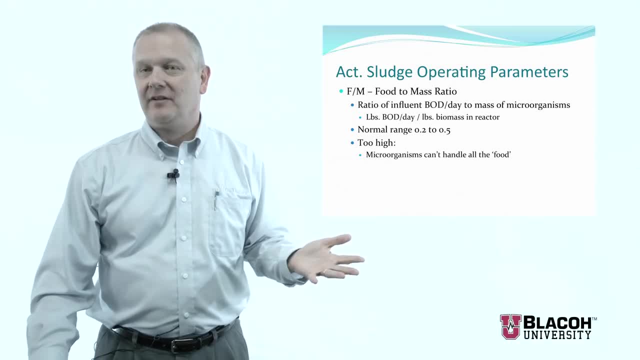 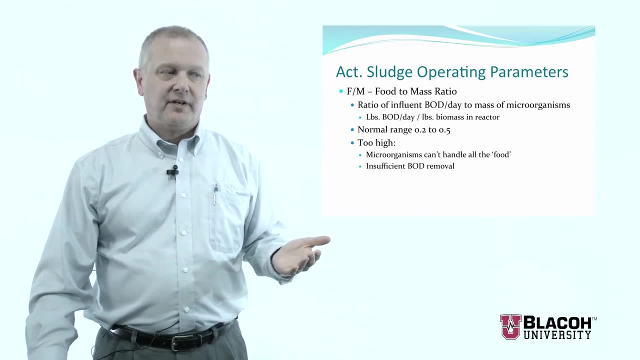 If it's too high, then the microorganisms simply can't eat it all. They can't handle it all and you won't remove all of it from the waste stream. You also get what we call viscous. It's viscous bulking, which basically I liken to fat bugs. 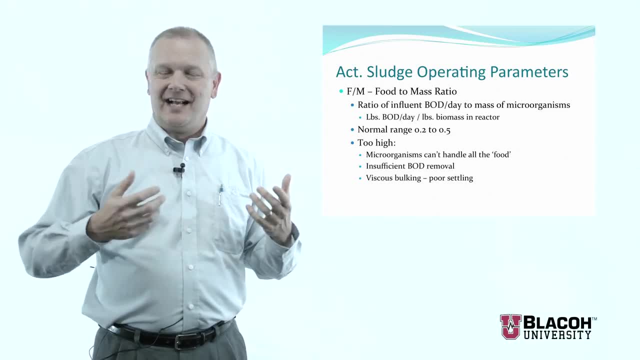 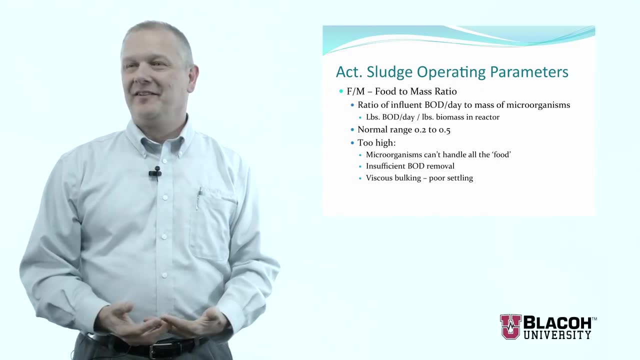 These microorganisms have eaten too much and it actually changes their specific gravity. It's not really fat- They don't get fat, but it's analogous to that- and they don't settle well in the clarifier and they'll even float sometimes and that doesn't work because you take the. 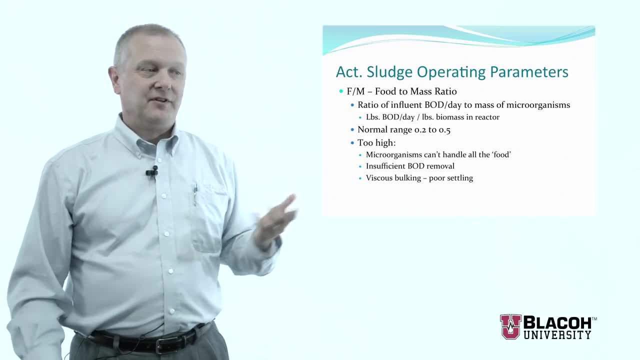 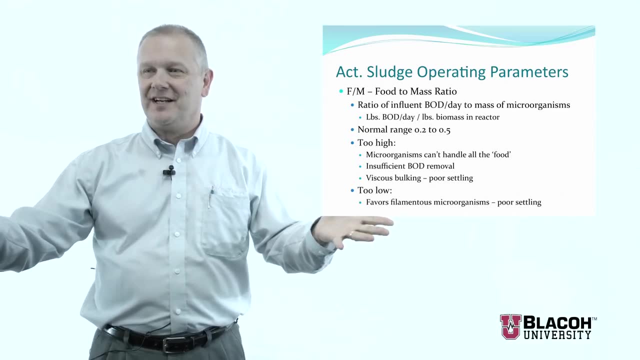 clear liquid off the top of the clarifier, But if it's too low, again you have problems with these filamentous organisms that are more efficient at getting what little food is there, and so they tend to predominate, and again you have poor settling in the clarifier. 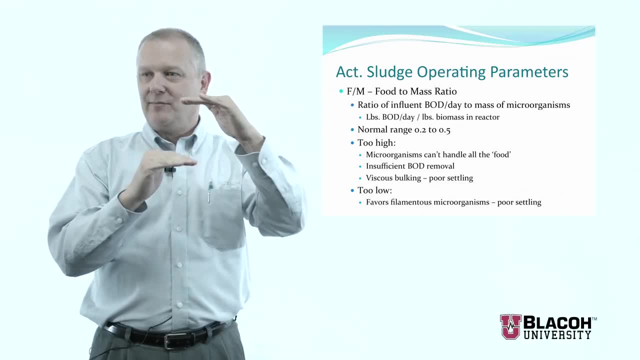 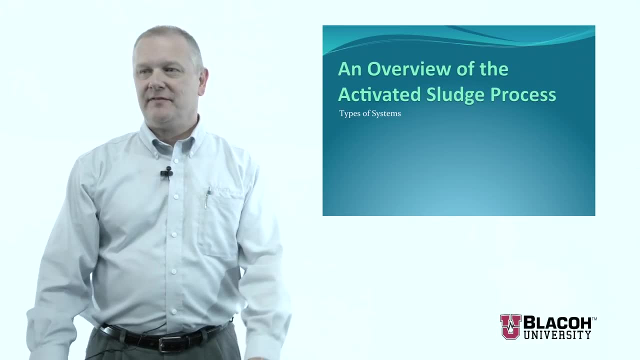 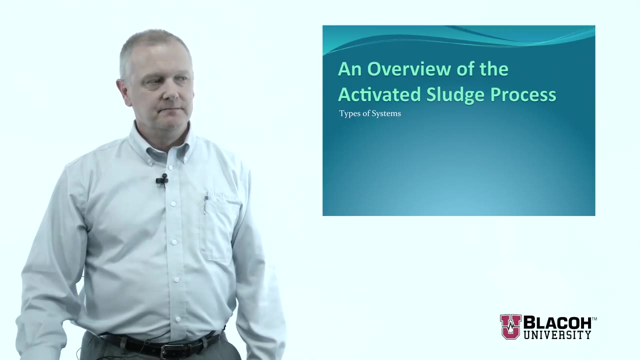 So you have to keep that food-to-mass ratio in a fairly stable range for this system to work properly. Let's look at different types of activated sludge systems in a practical standpoint. actually in plant designs The most common, for particularly in larger plants. 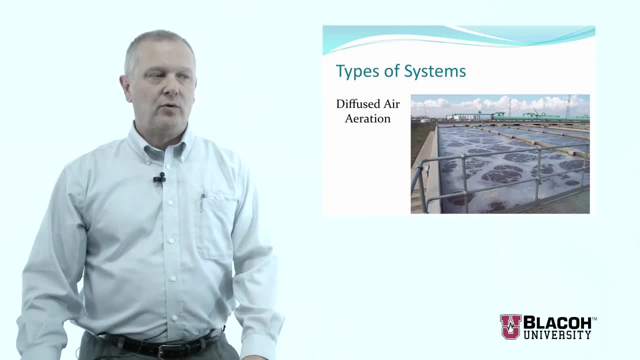 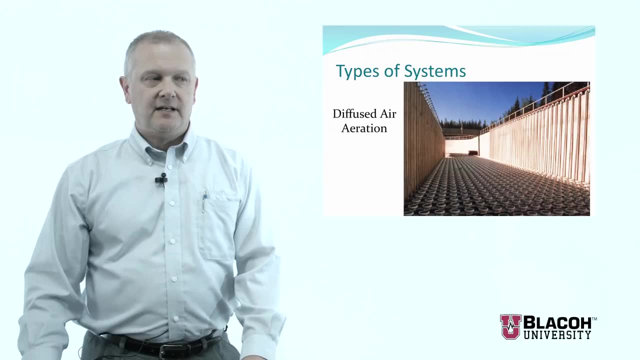 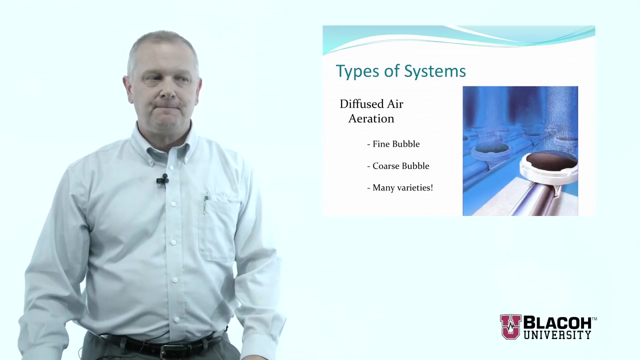 is a diffused aeration system where we bubble air from the floor up through the wastewater. Here's a picture of a tank that has a bunch of diffusers on the floor of the tank. It looks something like this, and there are many varieties of diffusers. 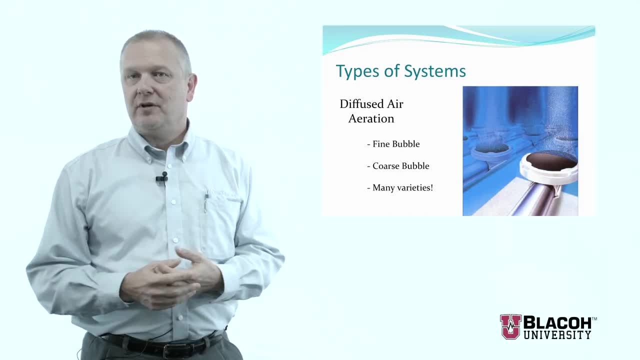 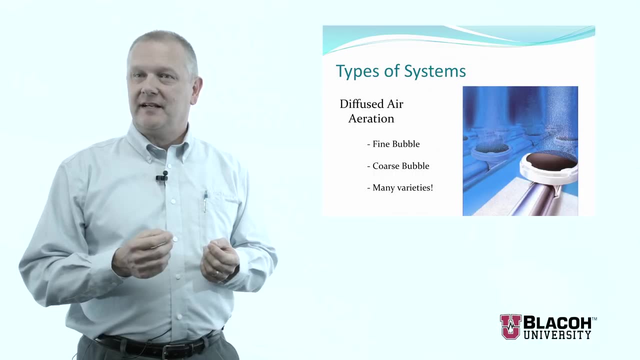 They can be designed for coarse bubbles, which do a better job of mixing but not so great a job of oxygen transfer, Or fine bubbles, which do a much better job of dissolving oxygen into the liquid but don't mix quite as well. 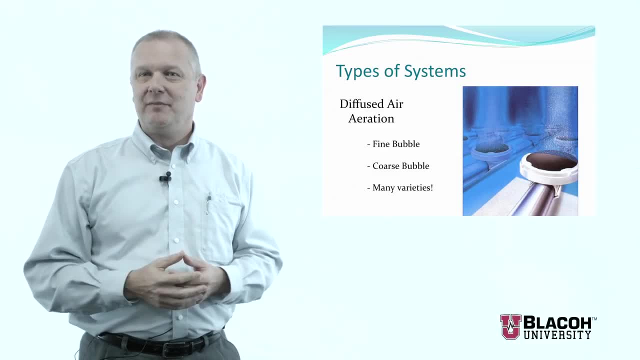 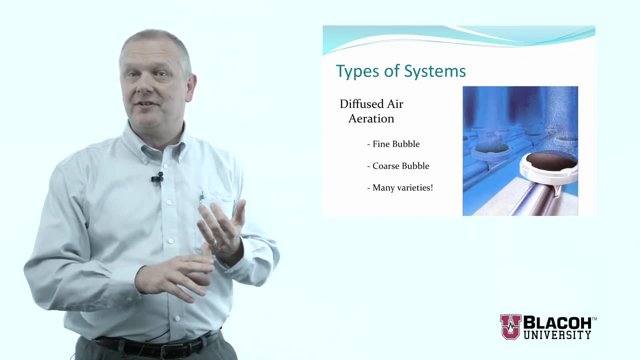 And there are many, many variations and shapes and sizes and designs that people have come up with, But basically they all just bubble air into the water And you need a blower or a compressor to push that air through the pipes and through these. 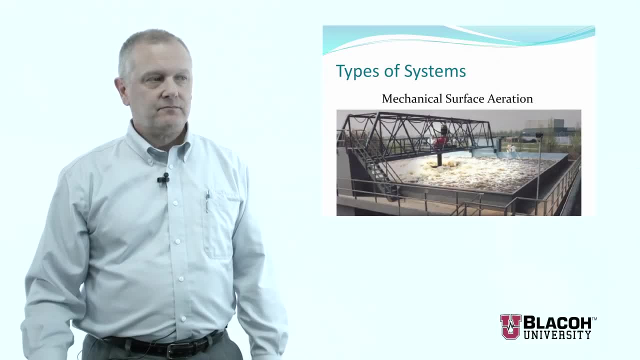 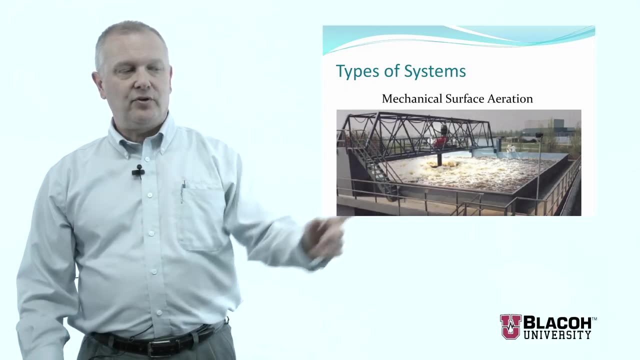 diffusers into the wastewater. The other type that's commonly used is some type of mechanical system. This is a type of mechanical system that's used in a lot of different ways. This is a type of mechanical surface aeration. Here you can see we have a vertical turbine aerator and it's splashing and churning the 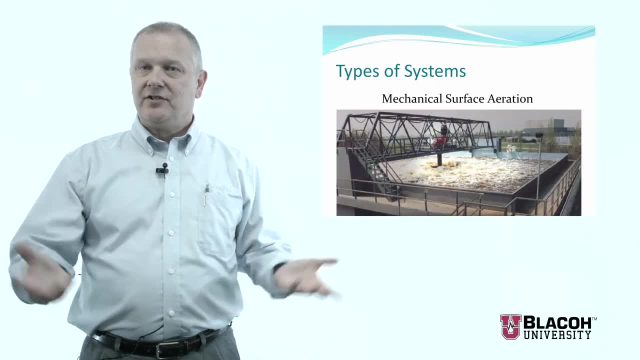 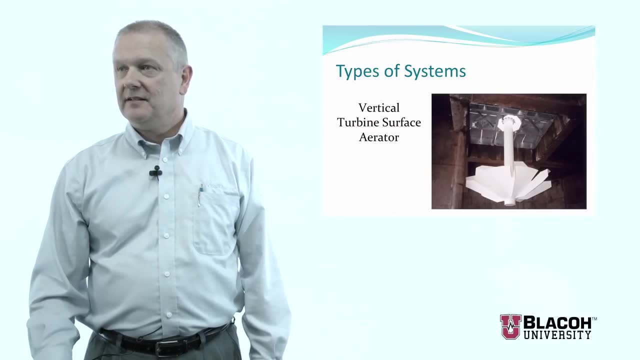 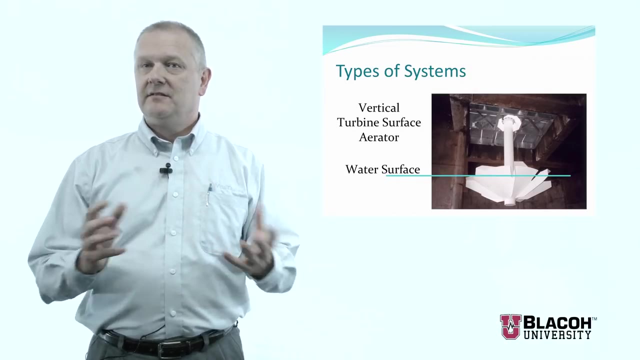 water. As it does that, the air gets entrained in the water and it dissolves oxygen into the water. This is what one of those looks like, when it's not submerged Water level's about there, It's only at the surface, but it acts to mix and aerate the liquid. 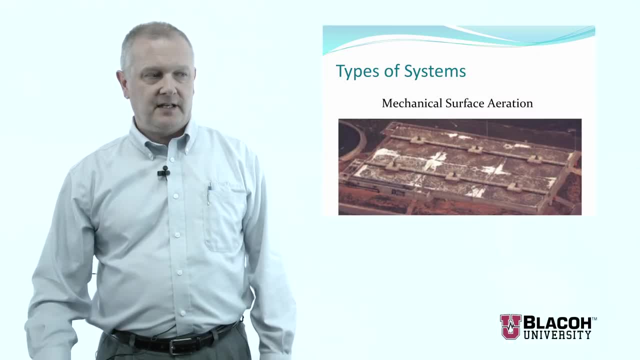 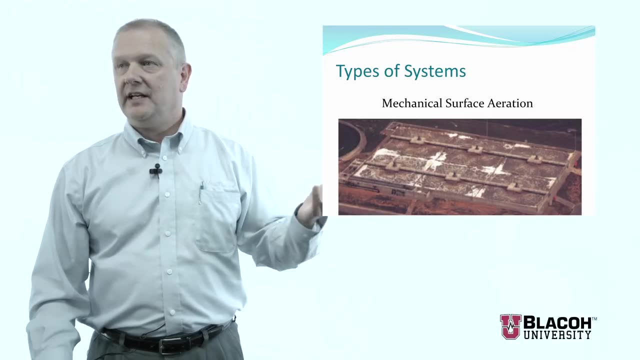 This is a type of mechanical surface aeration. Here you can see we have a vertical turbine aerator and it's splashing and churning the water. This is an example of a plant that's using those mechanical surface aerators. You can see it's just a big rectangular basin with six cells, each one with one of those. 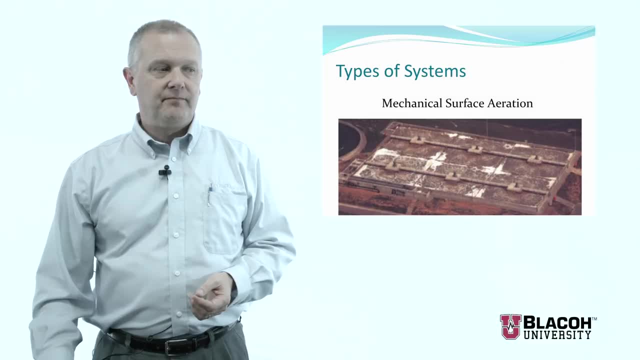 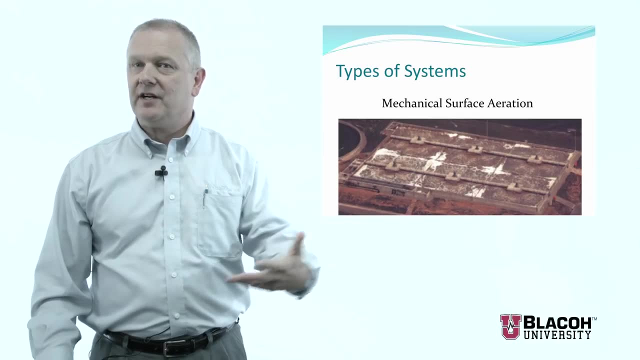 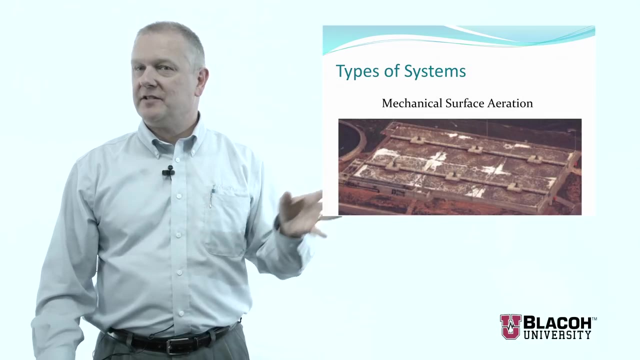 mechanical aerators in the center. This is actually not terribly common. Typically in rectangular tanks we use the diffused air systems and the mechanical aerators are saved for a type of design we call an oxidation ditch. that I'll show to you in just 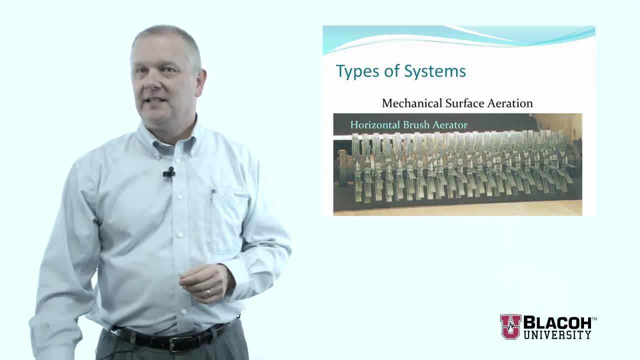 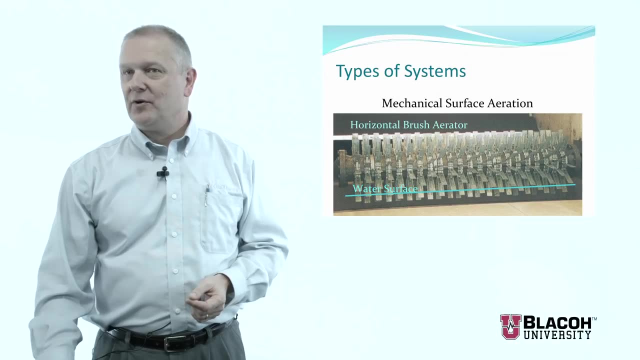 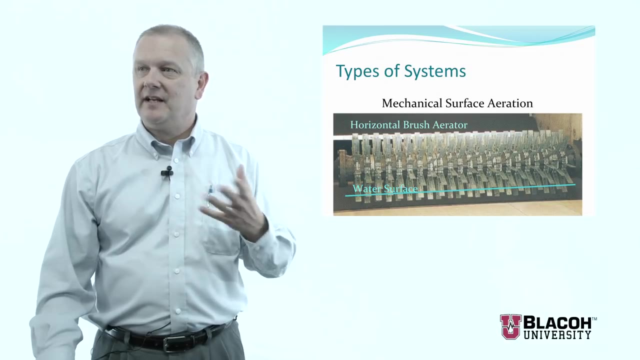 a minute. This is a horizontal brush aerator. This device spins around its horizontal axis there and it's partially submerged, so those paddles go through the water and basically do the same thing as the other one: They simply churn the surface up so they get a lot of foam and churning and air entrained. 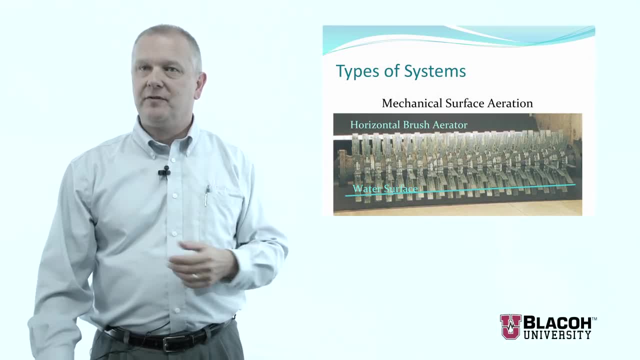 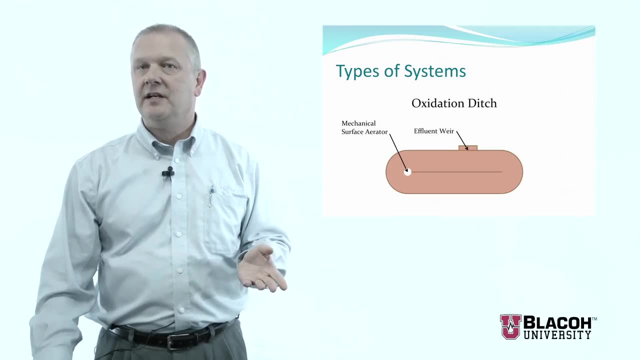 in the liquid and it also imparts a velocity to the liquid so that you can mix a tank. This is the oxidation ditch I was talking about. This is the most common application Or the common type of tank that's used with mechanical aerators. 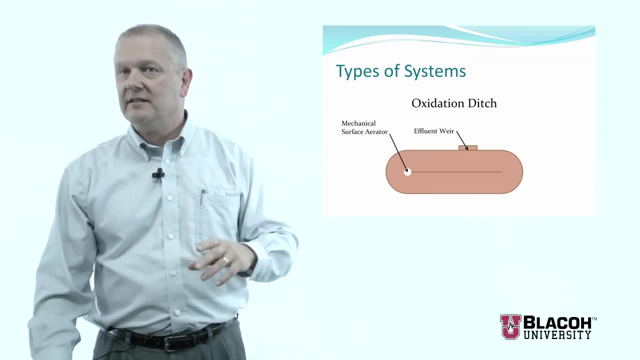 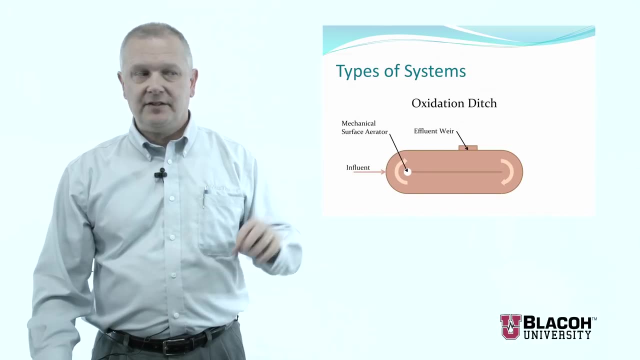 In this system the tank looks sort of like a racetrack. It's an oval and the influent comes in one end and you have either a vertical turbine aerator at the center of the circle at one end that will spin, or you put one of those. 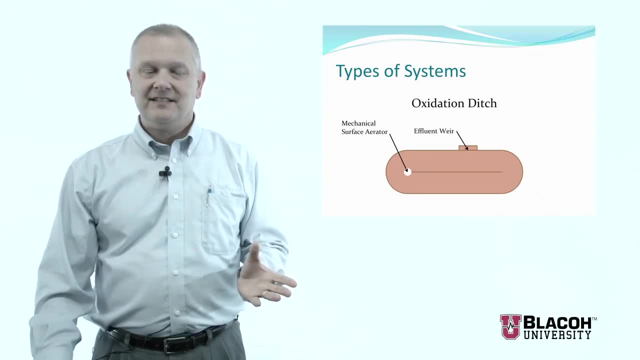 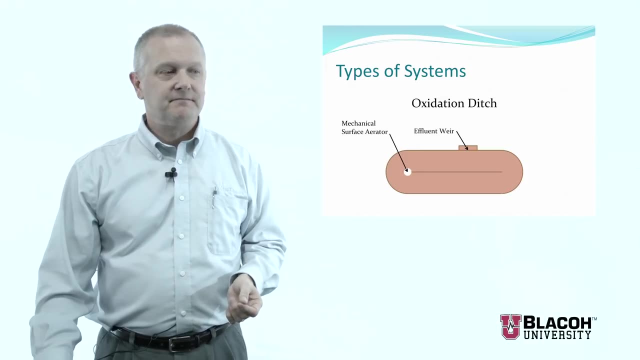 horizontal brush aerators on one side and it acts to move the liquid around this racetrack and aerate it at the same time. And of course, we have to then go to the clarifier and return our activated sludge back to the basin. 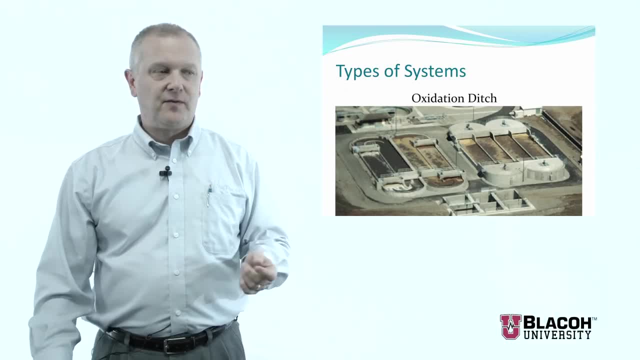 This is a photo of some oxidation ditches. I chose this photo because it actually has both types of mechanical aerators. On the right we have four vertical turbine aerators In the ditches. on the left we have six horizontal brush aerators. 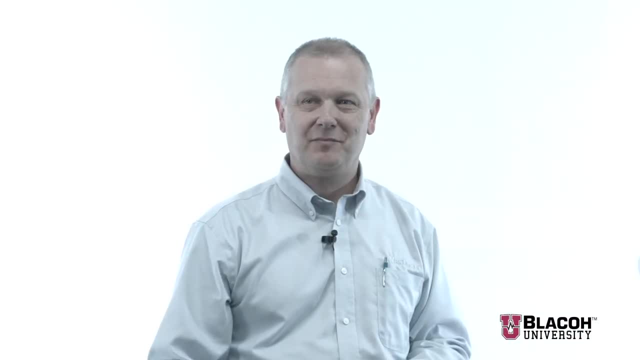 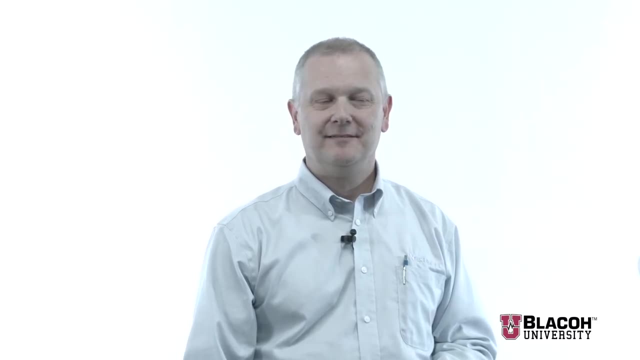 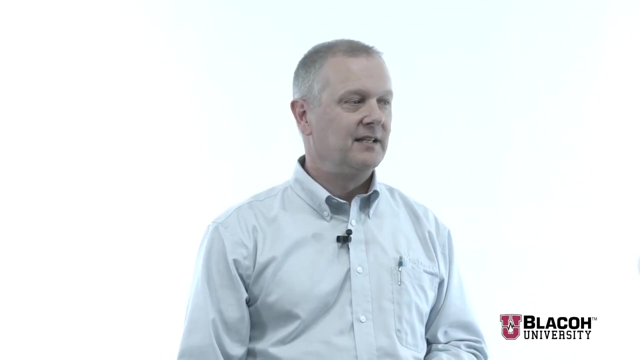 Obviously two different phases of development of a plant and expansion that occurred. Quick summary: Activated sludge is the most common secondary biological process used in wastewater treatment. It includes an aerated tank and a clarifier following and the sludge that settles in. 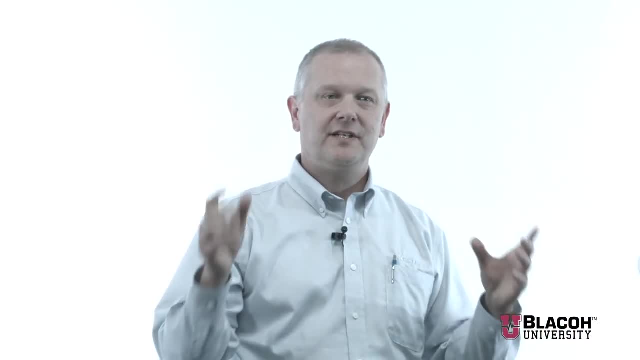 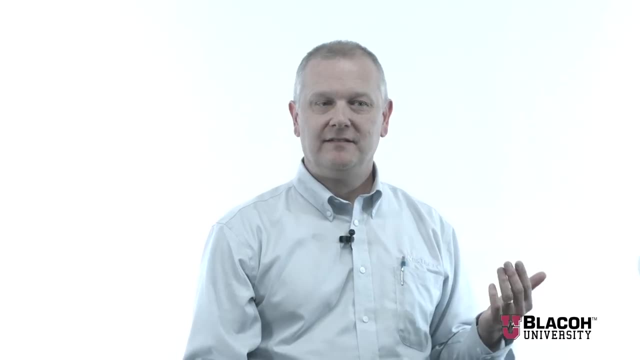 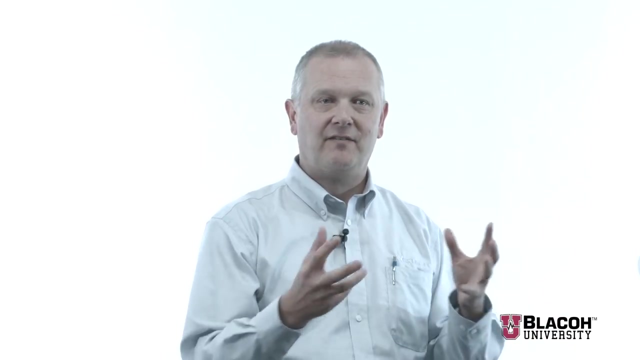 the clarifier is recycled back into the aeration basin to increase the amount of microorganisms to treat the wastewater. We talked about some treatment parameters that measure the effectiveness of the treatment process. Those were BOD- biochemical oxygen demand- Remember that's the amount of oxygen that's used up in breaking down that organic material. 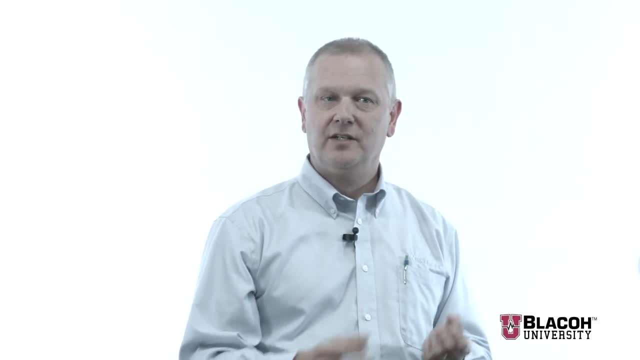 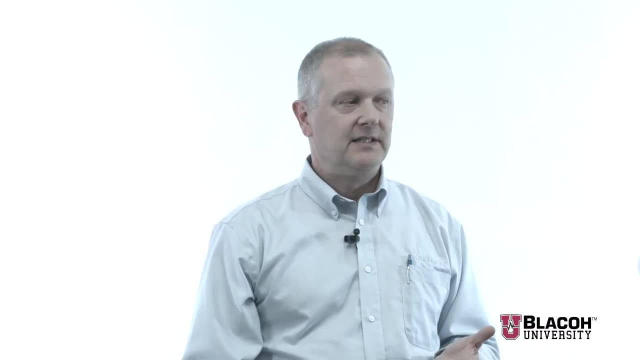 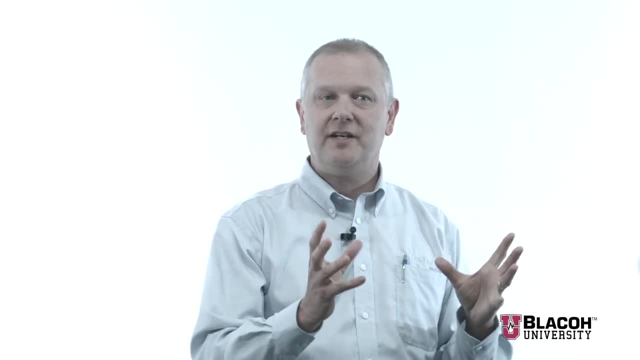 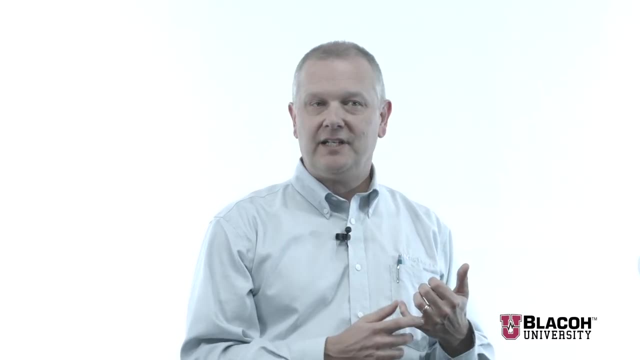 Mixed-liquor-suspended solids. That's just a measurement of the concentration of solids in the aeration basin. The dissolved oxygen concentration is critical to good growth of the microorganisms. The hydraulic retention time is important to give the microorganisms time to break down. 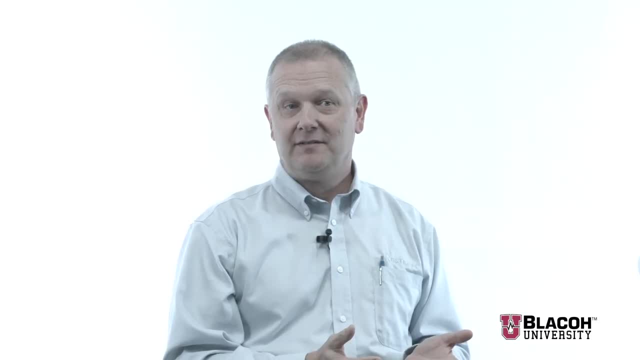 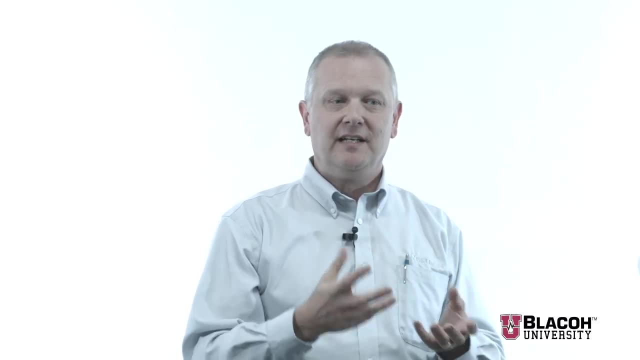 the waste, The solids. retention time is important to make sure we have enough microorganisms in the system. And finally, the food-to-mass ratio is just a measure of how many microorganisms we have versus their food supply, and we have to keep those in the right balance. 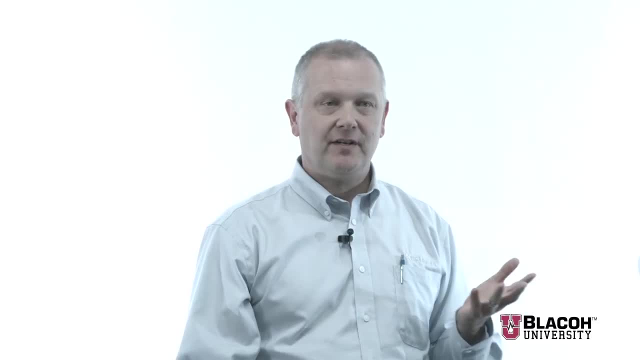 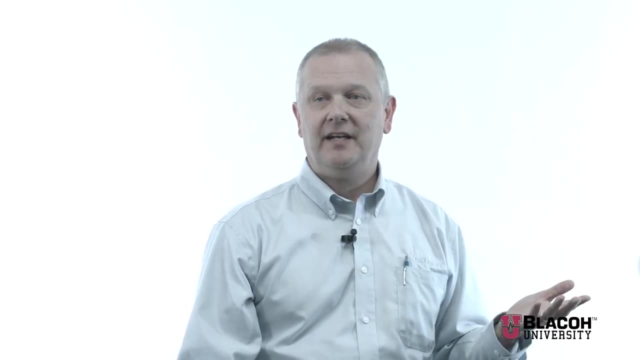 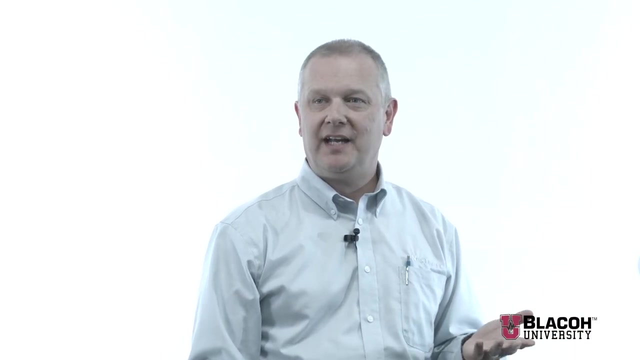 I mentioned a couple types of activated sludge systems. We have diffused air systems which can be coarse bubble or fine bubble and can accommodate basically any tank shape you want, because you can simply put the diffusers on the floor. You can have a very odd-shaped tank sitting in the corner of a wastewater treatment plant.